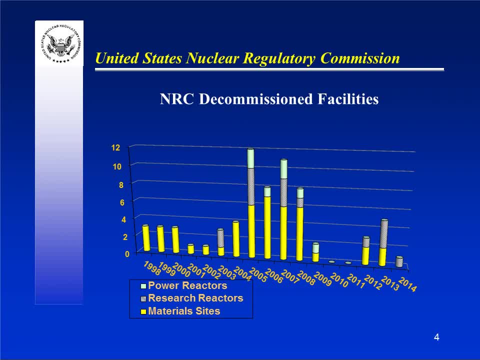 rules went into effect. We've decommissioned or terminated a license on over 80 materials- complex materials sites. We've done seven power reactors, although we've done 10 power reactors. in all, We've done approximately 13 research reactors. 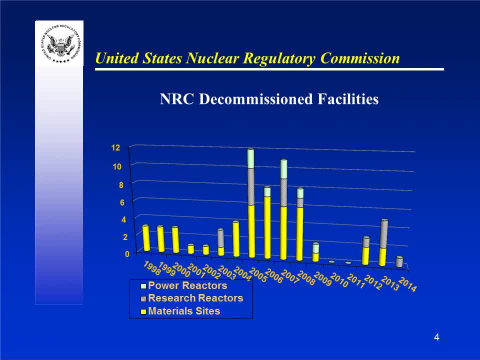 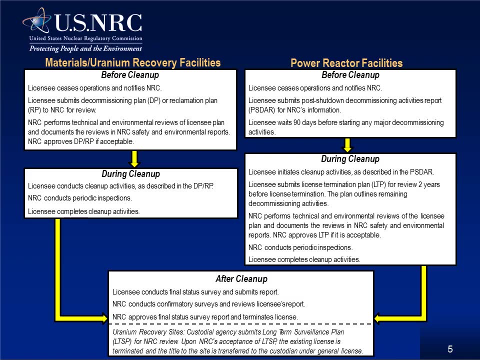 Actually, I want to make sure it's clear to you that we have two sets of regulations, one for material sites and one for power reactor facilities. Basically, in the material sites, they have to decommission the site fairly promptly, because there's no benefit in waiting. 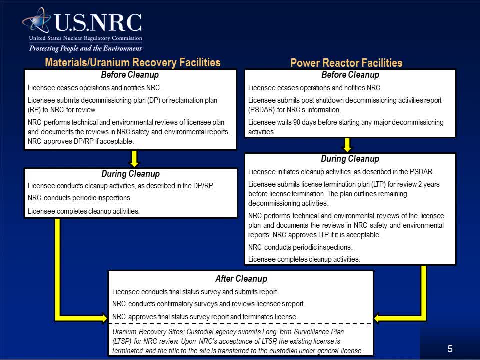 In most cases, those actually have a decommissioning fund which needs to be used. It's not wasted or squandered, so they get the decommissioning completed fairly promptly. With the power reactors, though, they have up to 60 years, and this is the general process. 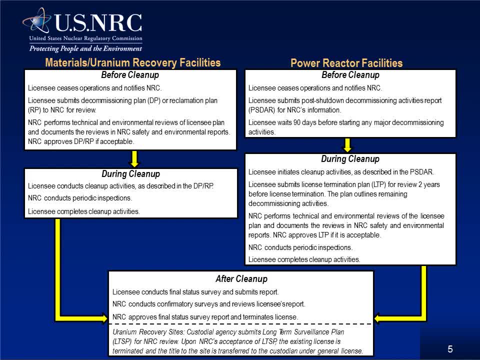 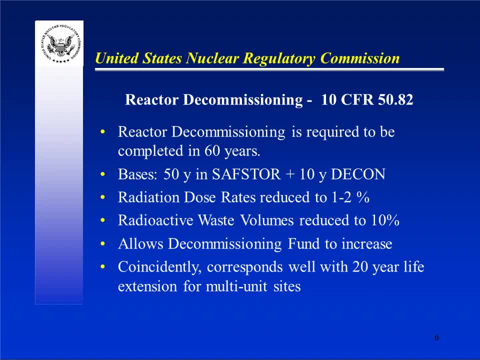 here, which I'll go into more detail. Like I said, the reactor decommissioning regulations are in Part 50.82.. It requires that the reactor decommissioning is completed within 60 years. The basis for that is you put the plant in. 50 years of safe store. In other words, mothballing. That's what we're going to do. We're going to put the plant in 50 years of safe store. In other words, mothballing. That's what we're going to do. We're going to put the plant. 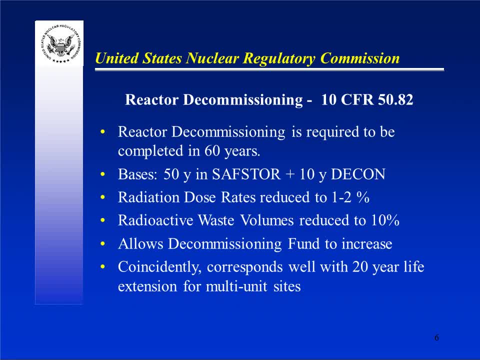 in 50 years of safe store After it's been mothballed for 50 years, and then they have about 10 years to complete the decontamination and go to decon. Now the safety results of this are that the radiation dose rates are reduced to about. 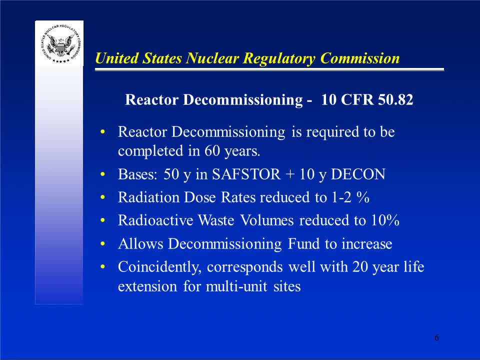 1-2% of what they were when the plant first shut down, so there's significant radiation exposure to be saved. Also, it's estimated the radioactive waste volumes can be reduced to about 10% due to radioactive decay of the materials in the reactor and its systems. 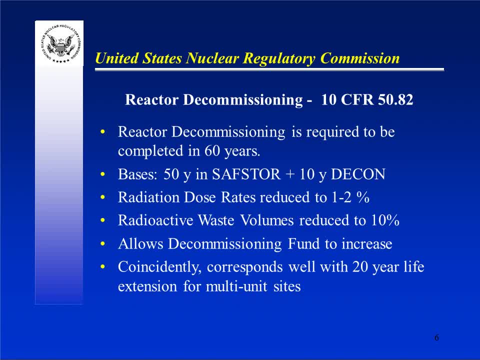 By coincidence this allows the decommissioning process to be completed fairly promptly, decommissioning fund to increase, since they're required to have a decommissioning fund all the time and with 50 years they can let it build pretty high. 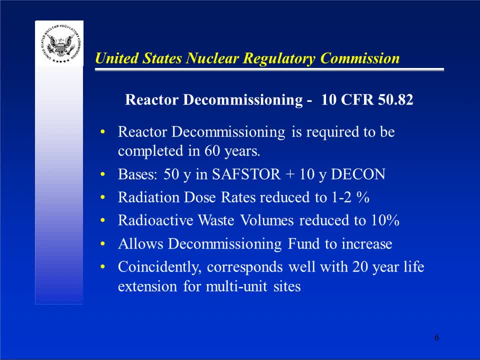 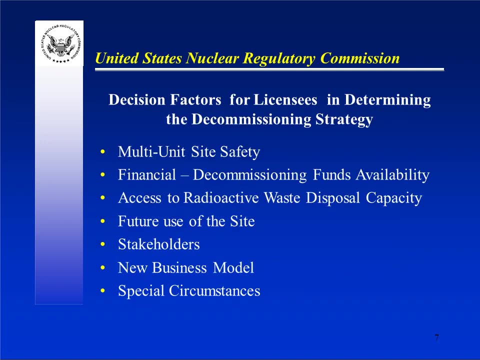 This actually coincides very well with the 20-year license extension that many of the power plants have and it's used extensively at multi-unit sites Decisions factors for licensees in determining the decommissioning strategy. the first one is multi-unit site safety and most of the sites in the US where there's more than 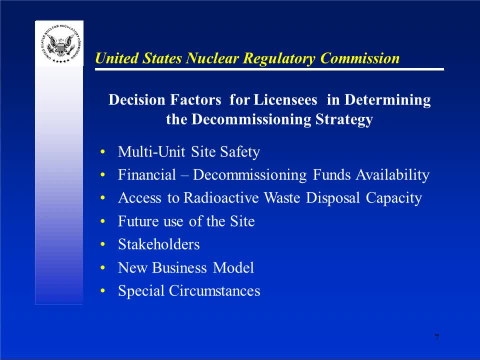 one unit. the first unit was built generally one generation or so before the others and so it shut down early. but they store until the other operating reactors are ready to be decommissioned. In this case we consider that a safety issue in the fact that the licensee can focus on. 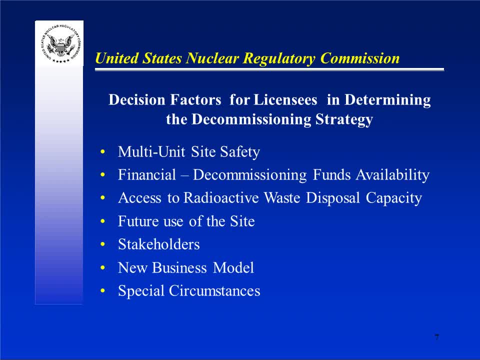 the operating units and not on the decommissioning unit. Part of the decision making is financial: whether the funds completely are available to complete all the decommissioning, and our regulations require that they have funds available for the radiological decommissioning, not the complete decommissioning as people think. 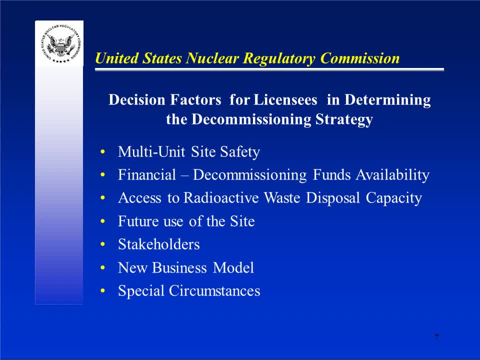 and we'll get into that a little bit later. One factor that other reactors have had in the past is access to the radioactive disposal capacity. In other words, is there a waste disposal site available? Back in the 1990s, some people may recall that Barnwell was closing to out of compact waste, so the 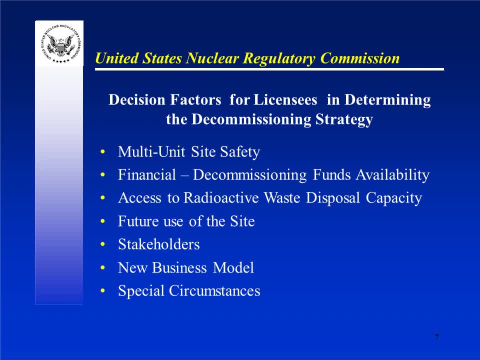 decision was to go ahead and properly decommission some sites so that they could remove the waste from the site and dispose of it. Another key factor is the future use of the site. Many of these sites are of great value to the utility. As a matter of fact, many of them build additional generating capacity on them, since there's 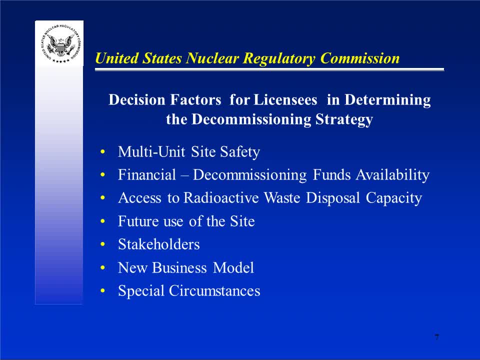 cooling water. There's already been an environmental impact, There's a statement done there and there's the infrastructure for the grid to produce the electricity out into the grid. Another important thing is the opinion of stakeholders in the local area and in the state, whether they want to have the site decommissioned right away or not. 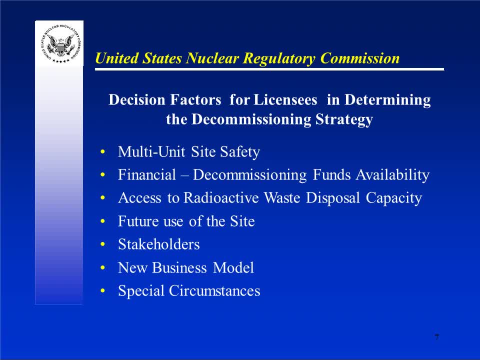 There's also a new business model out there in which a private company takes over the actual reactor license and decommissions the site for profit. The Zion Solutions has a I don't know. I don't know. They took over the Zion site a number of years back and they're probably about two-thirds. 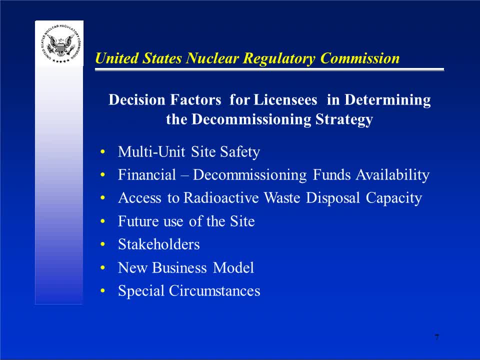 the way of completing the decommissioning at Zion 1 and 2.. And then there's special circumstances which may influence those decisions. For example, San Onofre is on land leased from the US Navy, and so the agreement for. 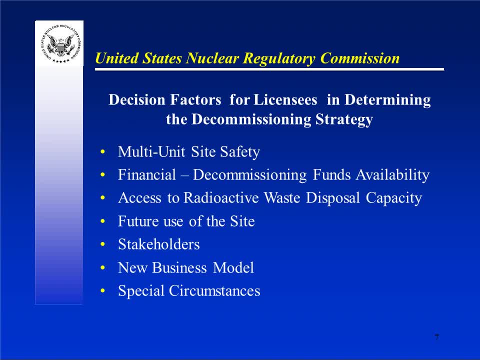 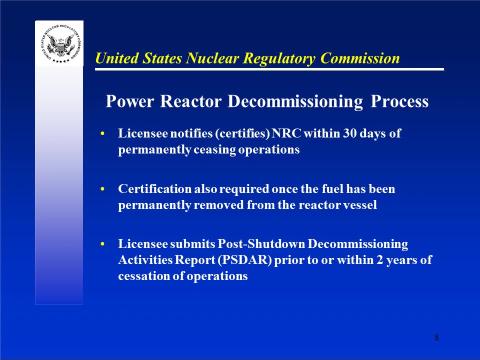 the decommissioning is in their agreement with the Navy and the Marine Corps for when they will decommission, when they shut down The power reactor decommissioning process is basically two certifications. First, the licensee tells us they're going to permanently cease operations within 30. 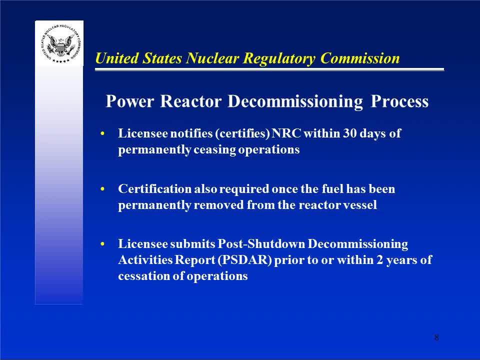 days, And then a second certification is required once the fuel has been permanently removed from the reactor. At that point they are no longer allowed or authorized by law to put the fuel back in the reactor and operate the reactor, so not restart the reactor after that point. 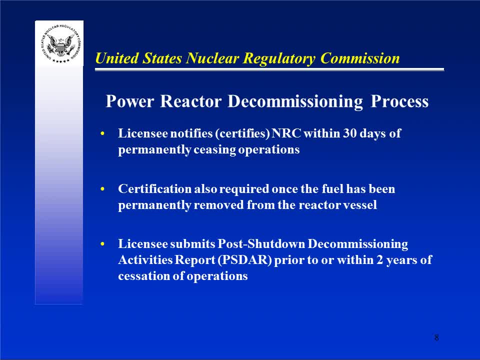 But this is a key thing for if you're thinking in emergency planning. After that, the licensee is required to submit to us a post-shutdown decommissioning activities report prior to or within two years of the cessation of operations, And we'll talk about that in more detail here. 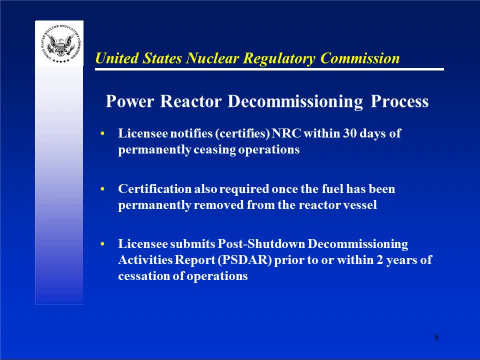 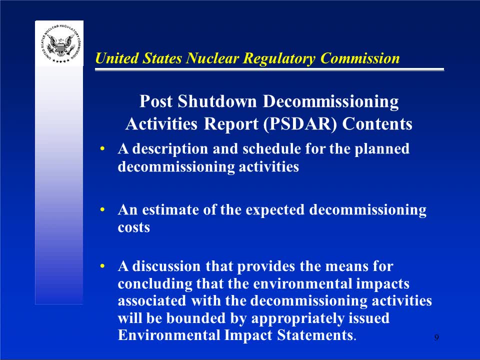 The PSDAR, as we would call it, is basically a description and schedule for the planned decommissioning activities. Are they going to go into decon, Are they going to the safe store? And what their actual plans are, what their decommissioning strategy is? 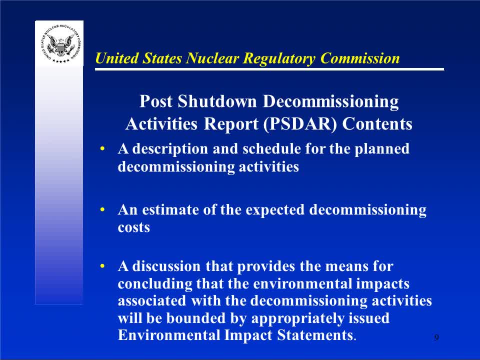 Thank you. It is also an estimate of the expected decommissioning costs and it's also to provide a discussion that provides the means for concluding that the environmental impacts associated with the decommissioning activities will be bounded by the appropriately issued environmental impact statements. 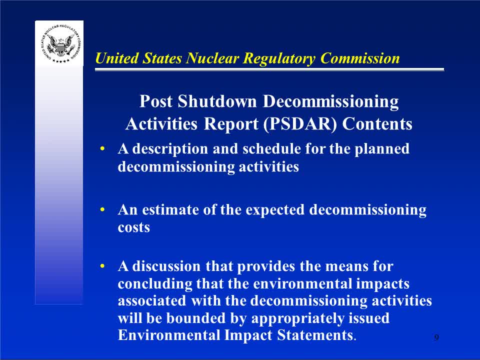 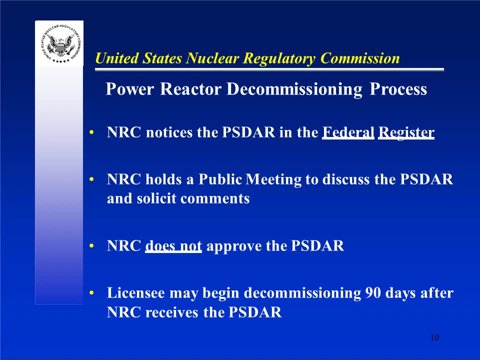 In other words the decommissioning. can the decommissioning be completed within the current environmental assessment for the site? Actually, with the PSDAR, we will notice it in the Federal Register. We will hold a public meeting. We will discuss the PSDAR and solicit comments from the public. 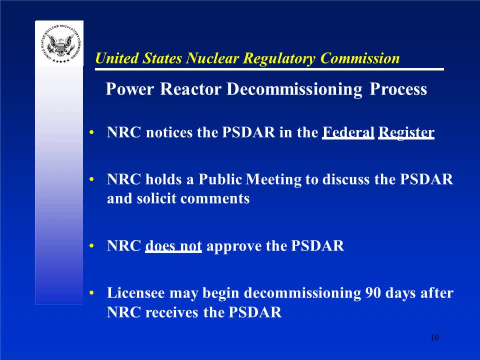 One of the key issues is what we do not approve: the PSDAR. It is merely a notification letter to us on their plan strategy and verification that they have the status of the funds and that they can remain within the current environmental impact statement to begin the decommissioning. 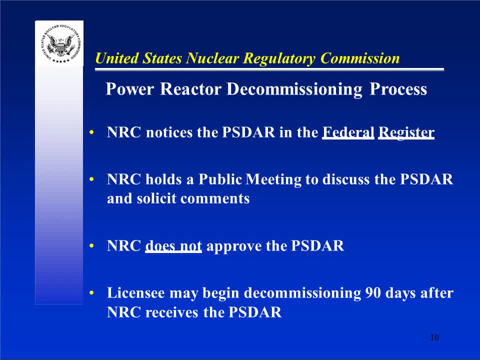 Keep in mind that they can do the decommissioning within their current license, So there's no need for any licensing. So this letter is mainly just a notification. However, we do have requirements for what the content of that letter is, and you can find: 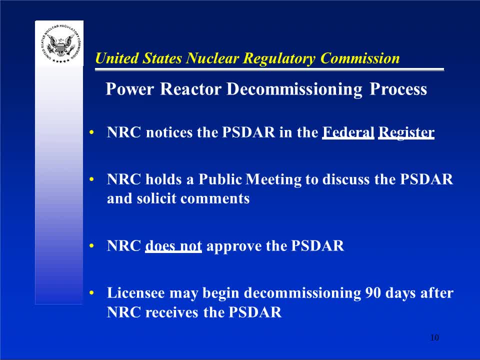 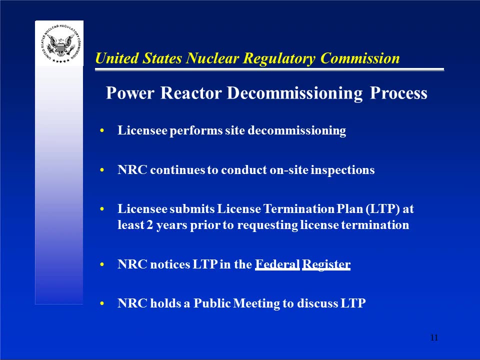 those in Reg Guide 1.185.. And, of course, in accordance with the regulations, they can begin decommissioning- major decommissioning- within 90 days after we receive the PSDAR. After that, the licensee will perform the decommissioning whatever schedule they have. 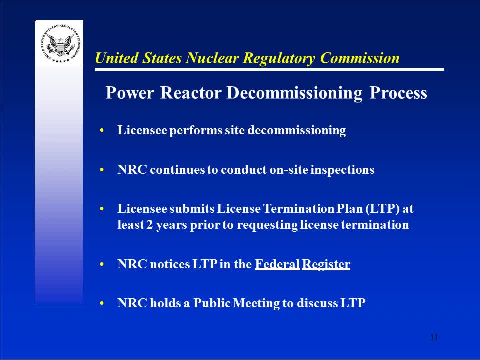 planned, We continue to conduct on-site inspections. during the decommissioning, The licensee submits what we call the license termination plan. The license termination plan is required to be submitted two years prior to requesting the license termination. So it could happen in year eight if they chose a prompt remediation, or year 58 if they were. 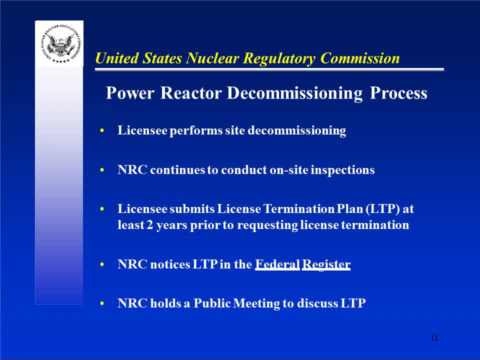 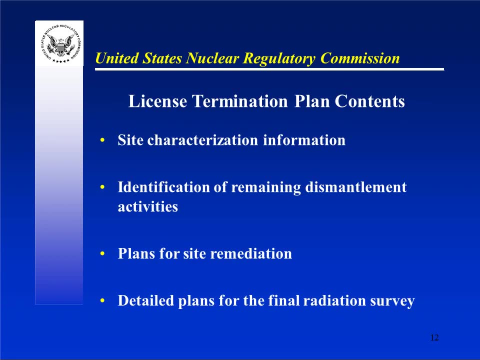 going for a safe store with a full 50-year safe store time. We will notice the LTP in the Federal Register and we will hold a public meeting to discuss the LTP. The LTP contents include all the site characterization information, identification of remaining dismantlement activities, the plans for site remediation and, of course, 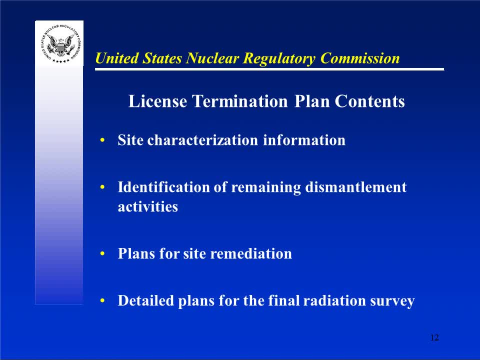 the key factor is the detailed plans for the final radiation surveys, because this is how they're going to demonstrate to us that they meet the dose criteria for releasing the site. And the dose criteria is for unrestricted use is 25 millirem per year plus all the 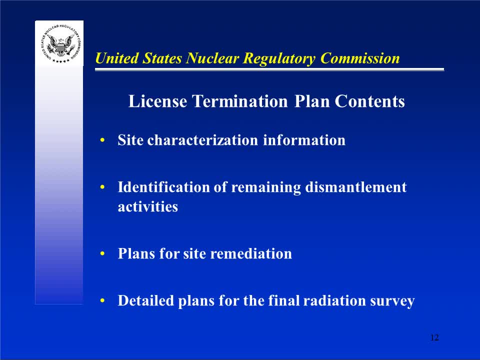 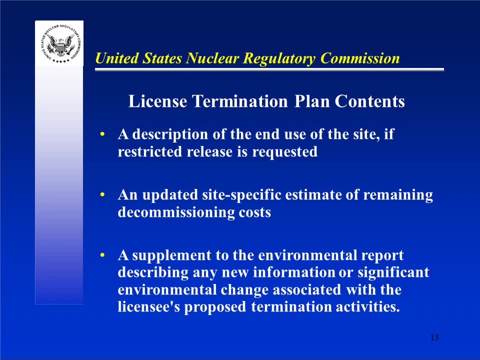 LARA actions. The LTP also contains a description of the end use of the site if restricted use release is requested. Now, out of all the decommissionings we have had in the country, none have had a restricted release granted, And so everything has been granted for or approved. like I, 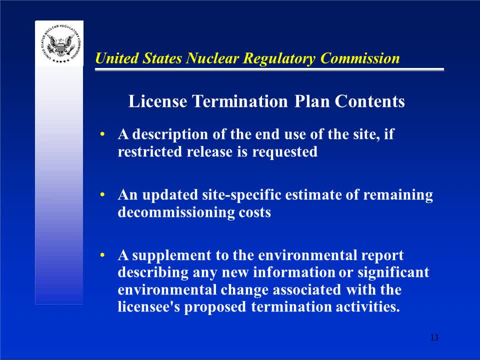 said licenses have been terminated for unrestricted release. In other words, the licensee or the owner of the property can use the property for whatever purposes they want to in the future. So keep in mind anything could be built on that, including up into a farm, depending. 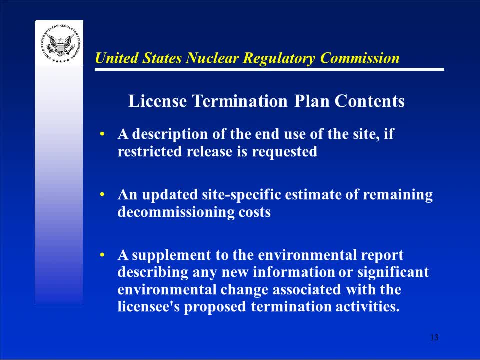 on what the licensee wants to do. It also requires an updated site-specific estimate for the remaining decommissioning costs and, of course, a verification on the environmental report. again, Okay, As far as the NRC review of the LTP, we conduct an acceptance review. We perform. 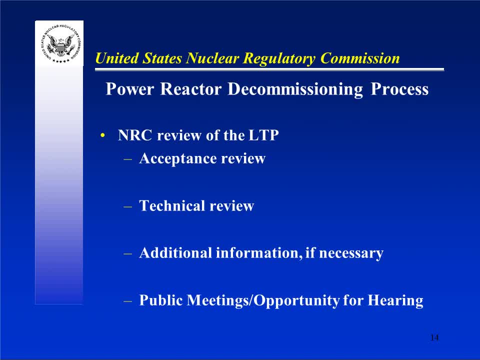 a technical review, which generally takes about a year. We request additional information if we need it And, of course, we will conduct public meetings and there's also an opportunity for hearing on the LTP. We approve the LTP by amending the license. The licensee will then perform all the remaining. 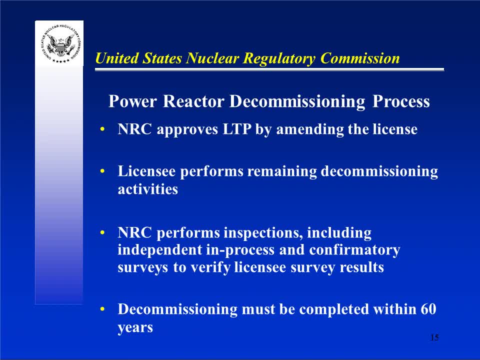 decommissioning activities. We will continue to perform inspections, including independent in-process and confirmatory radiological surveys, to verify the licensee meets the survey requirements and they meet the limits established for the release of the facility. Again, the decommissioning must be completed within 60 years. 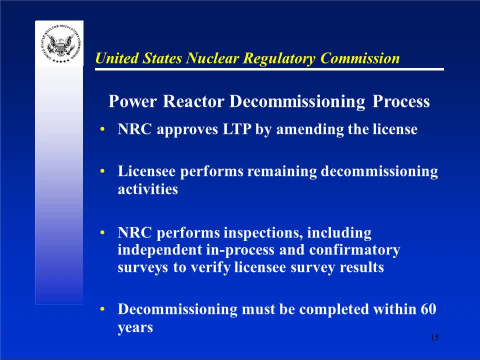 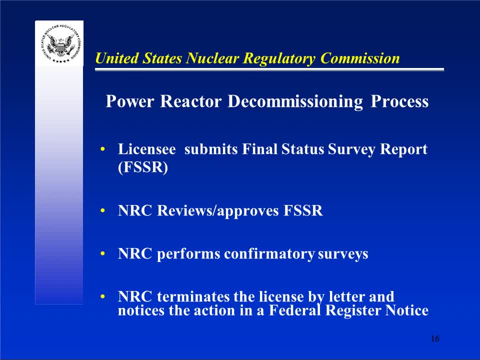 As far as the final parts of the process, the licensee will submit their final status survey reports to us. We will review and approve those final status survey reports. We will may or will have – will compile all those final status survey reports. We will conduct. 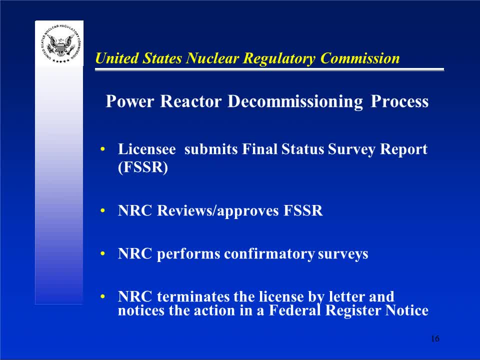 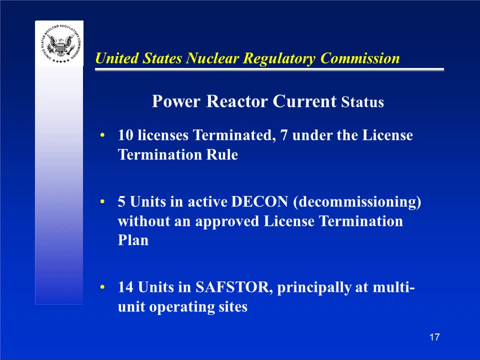 a review and approve those final status survey reports. We will – may or will have – will complete more confirmatory surveys and we will terminate the license by letter and by notices and of the action in the Federal Register notice. so far we have terminated the licenses on ten power reactor facilities, seven. those were done. 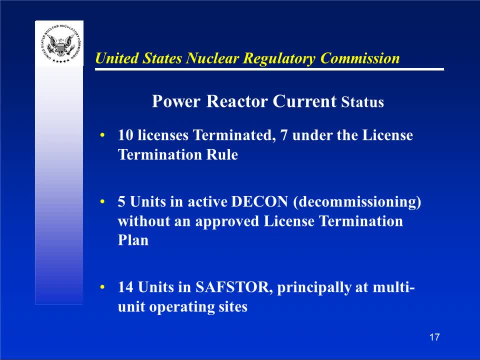 on the current license termination rule. under the current regulations, there are currently five units in active decontamination and they do not have an approved license termination plan because they are not anywhere close to having the license termination requesting the termination. we do have two license termination plans we are currently reviewing, and so we are very 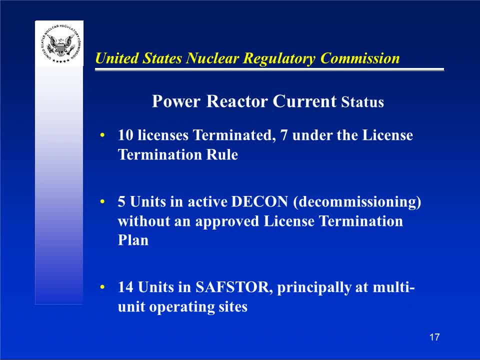 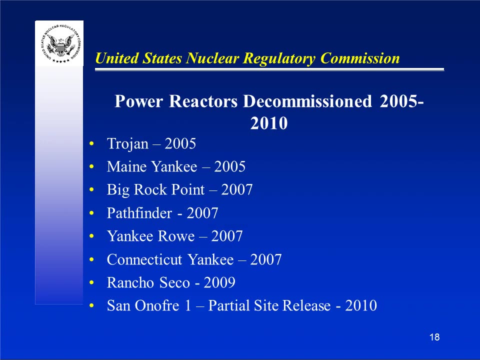 active in that area. right now, there are 14 units in safe store, and most of these are at multi-unit sites that have operating units. these are the power plants that were decommissioned from 2005 to 2010 and they were scattered across the country. 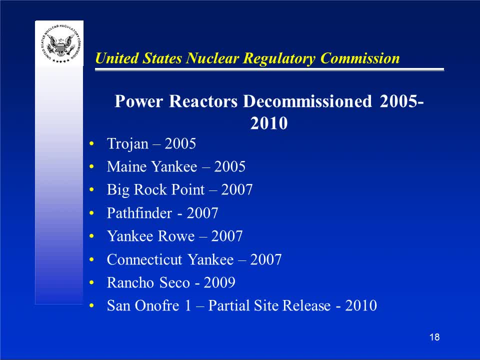 and invariably all of them were one unit facilities I had put on here. San Onofre unit one, because we granted a partial site release in 2010 and at that point San Onofre two and three continued to operate and San Onofre two and three. 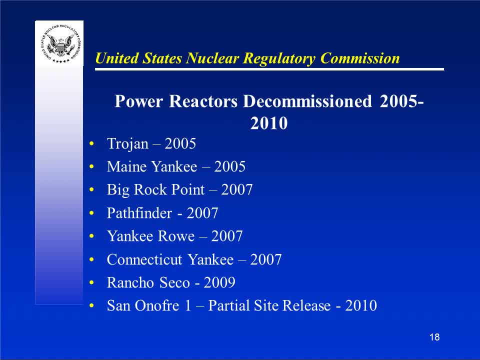 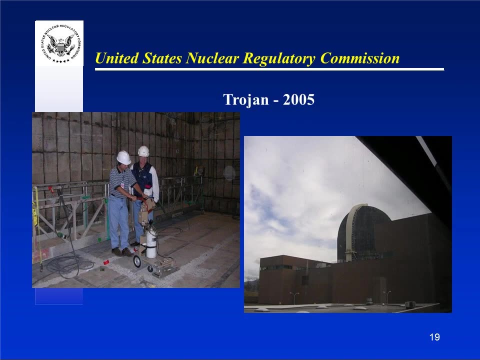 have shut down the actual material of San Onofre. one is the reactor vessel which is packaged and ready for shipment and on-site. this is- I thought I'd show you a few pictures. this is Trojan, which was. the license was terminated in 2005. on your left is a picture of us performing. 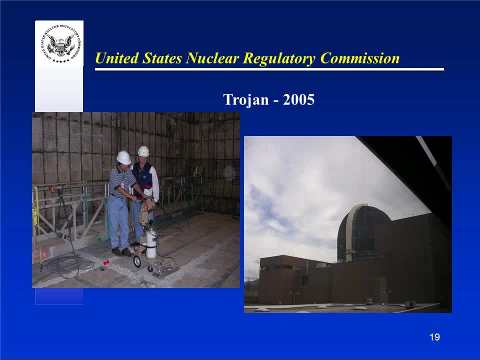 confirmatory surveys. and that is in the bottom of the, the former reactor spent fuel pool, which housed 15 years of operating spent nuclear fuel, so it can be decontaminated, it can be cleaned up. on your right, though, is the picture of Trojan when we terminated the license. as you can see, the 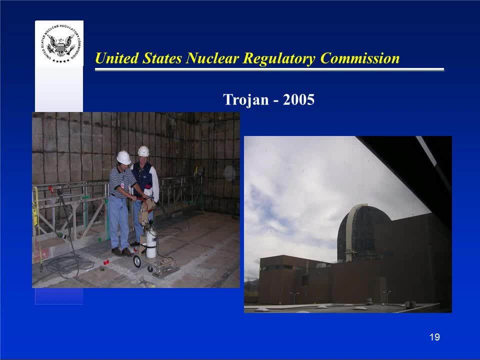 container containment building still there, the turbine building still there, the auxiliary buildings there. everything has been gutted with the from a radiological standpoint and this was their plan all along: was to leave the structure in place because once the radiological work is completed, we can terminate the license and they can do the deep demolition of the buildings. 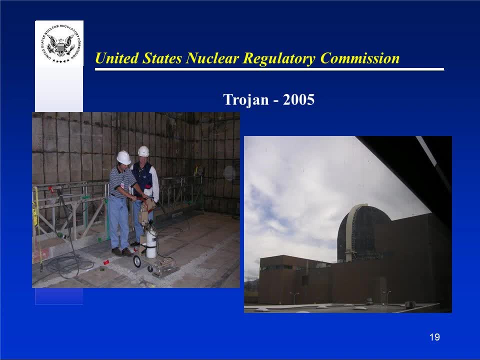 whenever they choose to. so they've chose to this model. they chose to decontaminate everything, terminate the license and then recycle as much more metal out of the facility as they could clean metal. this is a picture of Maine Yankee. on your left is the site as it looked when the plant was operating on. 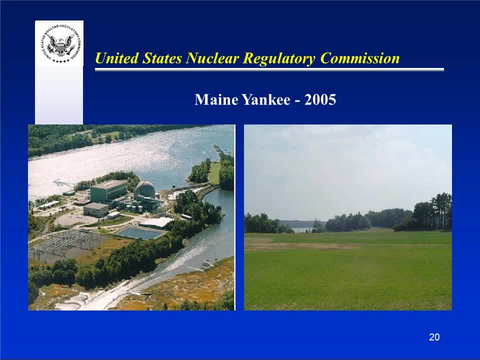 your right is a picture of the green field as they left it, and they actually removed all of the containment structure and buildings to a depth of about eight feet, and then we verified that the remaining structure was clean, hello contaminated and was allowed to terminate the license at that point. but 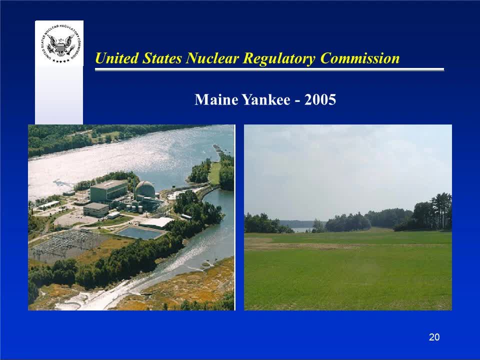 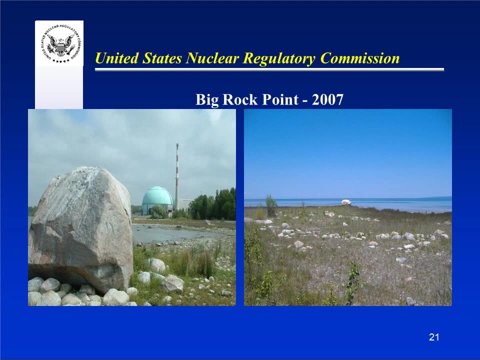 the site was green fielded. this is a picture of Big Rock Point, which is in northern Michigan. on your left is the picture of the Big Rock and the nuclear plant in the background. the picture on the right is a picture of where the plant was. as you can see, it's been returned to. 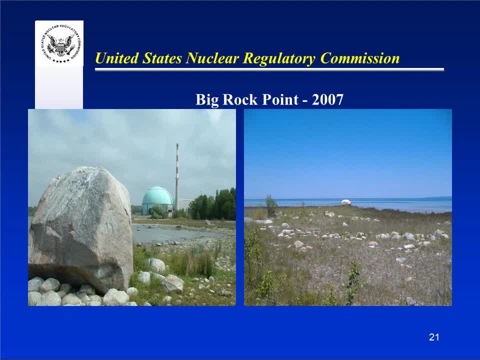 natural terrain along Lake Michigan and that's looking at the Big Rock. the Big Rock was a important to the Native Americans up there in northern Michigan because it told them when to turn to the right and head towards Canada during the summer and then when they returned to Traverse Bay for the winter, they would turn left. 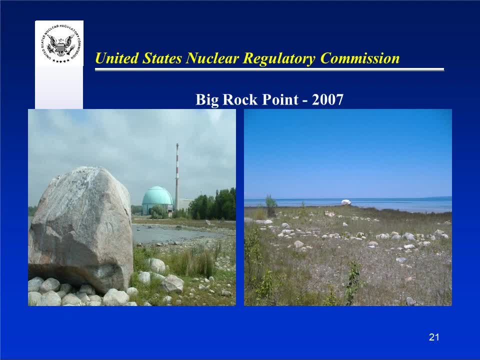 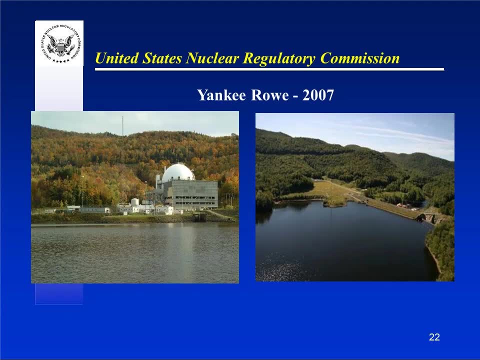 at the Big Rock. it's. that's the significance of the Big Rock. this is Yankee Row. we terminated the license in 2007. you can see it's been green fielded on your right, though I wanted to point out that that is a dam that has been in place a. 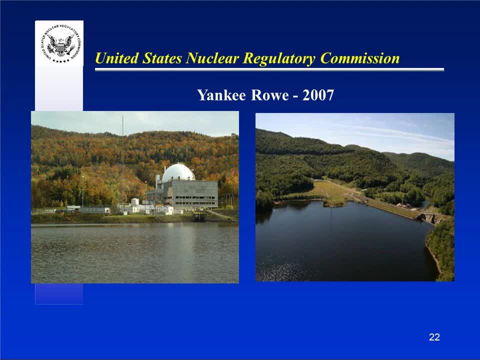 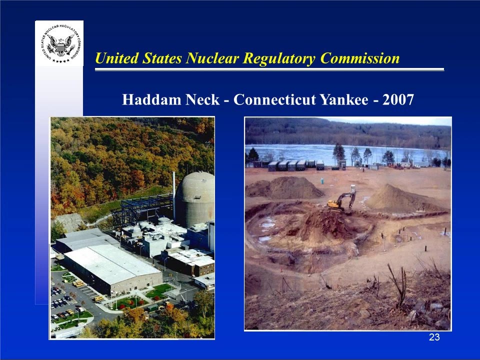 small hydroelectric dam that's been in in place for over a hundred years, so it outlasted the reactor plant. the next picture is Haddam Neck, also known as Connecticut Yankee. the license was terminated in 2007. they chose to go to green fielding. that's the Connecticut River. you can see the license is now in the. 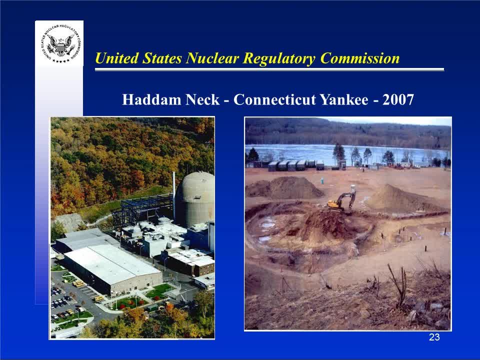 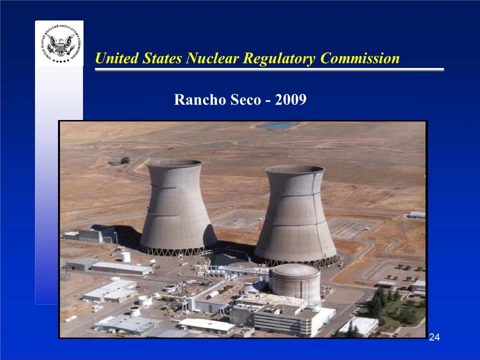 ground. you can see they were back filling here because they removed all the structures down to about six to eight feet below grade, and so now they're back filling here. on the right, this is a Array of Moseko. we terminated the license for the reactor back in in 2009. 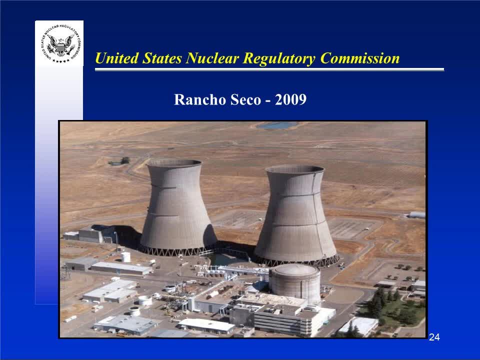 with all these facilities. I want to point out again that there is a spent fuel facility on site housing the spent fuel and drive storage. so when we terminate these licenses, we just So. when we terminate these licenses, we just generally shrink it down to just the the remaining spent fuel facility. this is 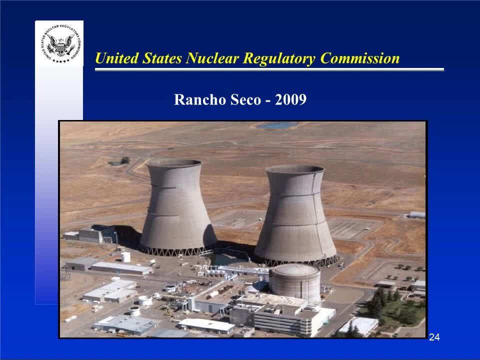 like I said, this is Rancho Seco, near Sacramento. their model was to decontaminate the plant, similar to Trojan, which they did, and so all the structures are left behind. there's not any radioactive materials associated with them, and I was just there this past summer and it looks basically the same. 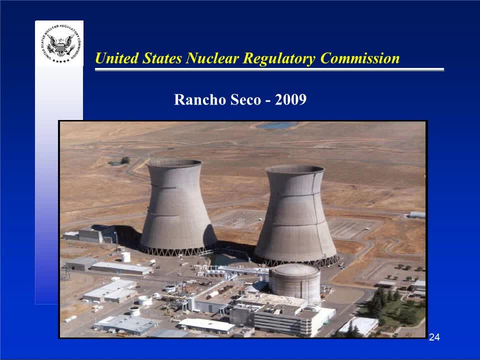 the utility has not spent any money knocking down any of the facilities. even the cooling towers are still there. the only big difference is where you see all that brown ground out there. that's now all vineyards. it was owned by somebody else who put in it's all Zinfandel grapes, is what I understand? that a whole 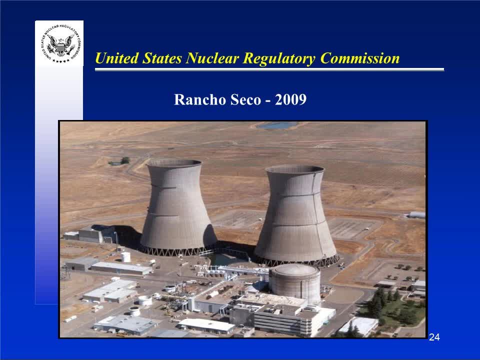 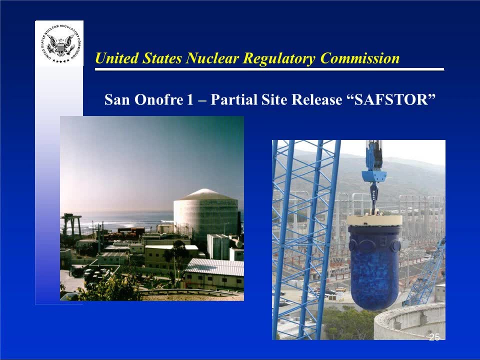 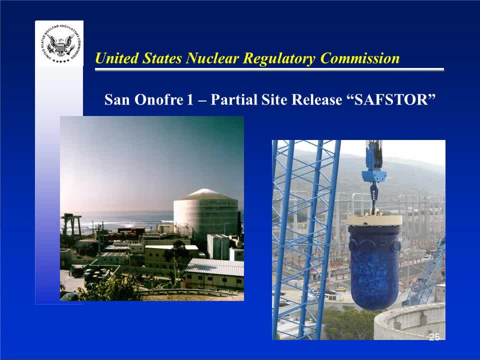 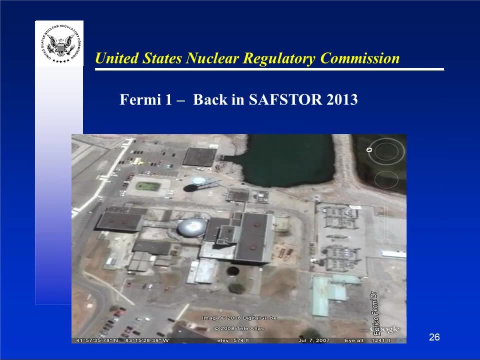 the only thing that that remains on site right now. it is packaged and ready to go for ship but to be disposed of when they get around to it. this is Fermi one. I mentioned to you before that they had sixty years to complete decommissioning. Fermi one has been going in and out of deacon and safe. 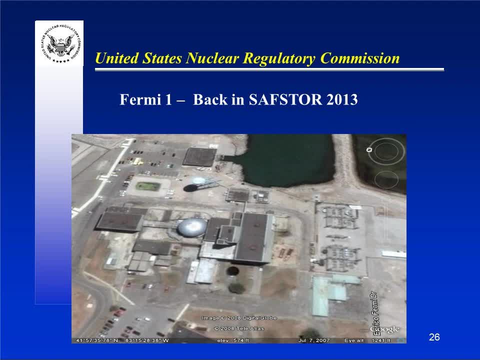 store over the last house eight, thirty, forty years and it They've removed most of the materials from the plant with the exception of some waste tanks and a couple valves or pipes, but in essence it's about 90, probably 95 percent complete. 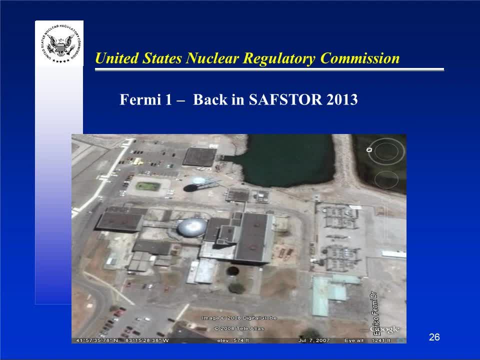 The reactor vessel's gone, all the reactor systems are gone and of course the spent fuel pool's gone, But they're back in safe store. They like to let the decommissioning fun grow and let interest rates grow. This is Humboldt Bay. 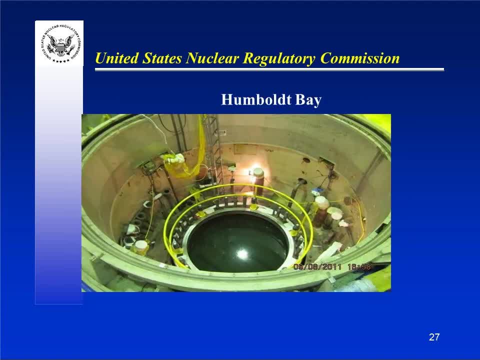 We currently have the license termination plan in for them. This is looking down on the dry well into where the reactor vessel is. the smaller rounder is the reactor vessel. They are just now completing segmenting the reactor vessel into small parts so it can. 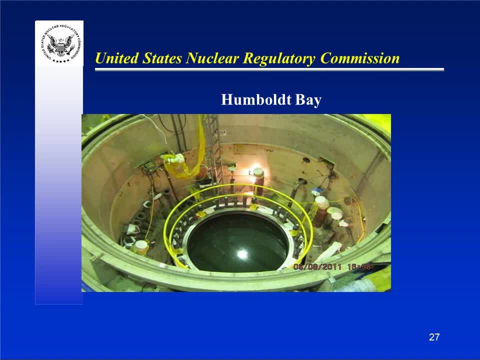 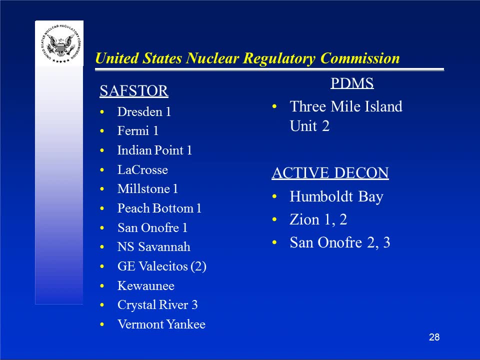 be shipped off. This is the list of current reactors in decommissioning. In the last year, Kewaunee, Crystal River and Vermont Yankee All shut down and notified us that they were going to be going into safe store. 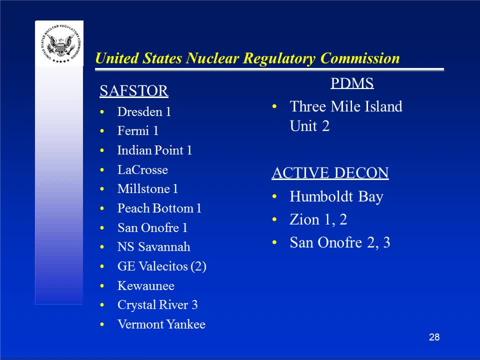 On your right, San Onofre 2 and 3 also shut down in the past, in 2013,- but they're going into an active decon stage. We have also in our- I guess I hate to call it- fleet of reactors, but we also have Three. 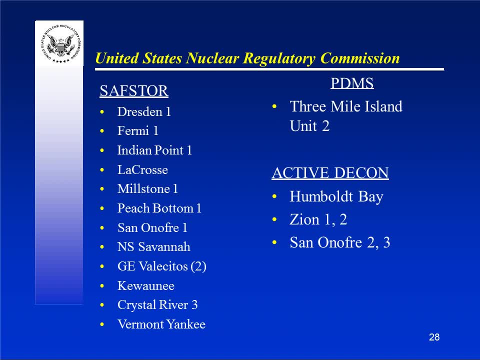 Mile Island Unit 2, which is in a special state called post-defueling monitored storage. Basically it's in San Onofre, That's San Onofre, That's San Onofre, That's San Onofre, It's in safe store. 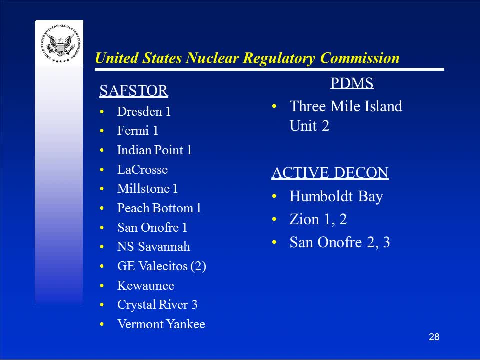 It will be for quite a long time while it continues to do decay, even though most of the damaged fuel is removed from it. I'd like to turn it over to my colleague, Bob Koehler, who's going to talk about emergency planning. 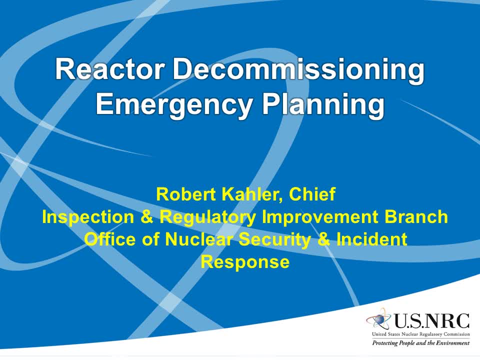 Hello everybody. My name is Bob Koehler. I'm the branch chief with the Inspection and Regulatory Improvement Branch in the Office of Nuclear Security and Incident Response. Essentially, my branch is responsible for maintaining oversight of the nuclear security and incident response. I'm also responsible for the inspection program emergency preparedness at commercial nuclear 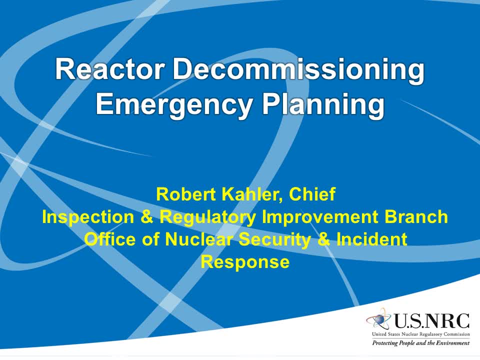 power plants and also for doing the rulemaking and guidance emergency preparedness for commercial nuclear power plants. I'd like to talk a little bit about what happens with a site once it gets into decommissioning, with regard to emergency preparedness at the site and also its interfaces with the off-site. 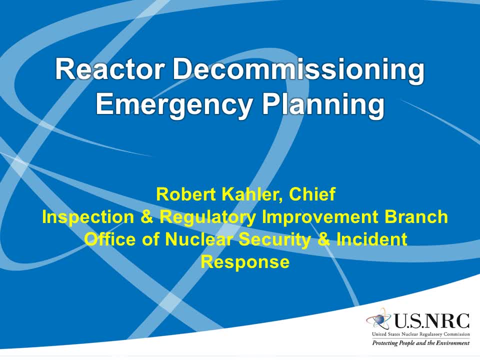 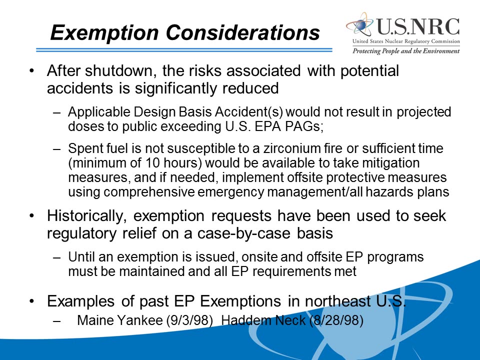 agencies who would be expected to respond to a radiological event at the site. Okay, Well, the first thing I'd like to talk about is that, as a plant is going into a decommissioning stage, they are looking at being a part 50 license, as we call it. 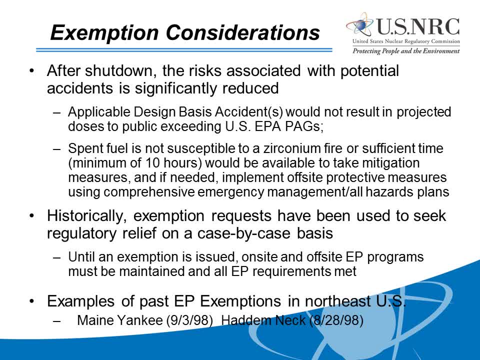 For emergency preparedness. there is no change in the status of how we look at them with regard to emergency planning. They do indeed have to continue to meet all of the regulations as if they were an operating nuclear power reactor. That has a lot to do with part 50.. 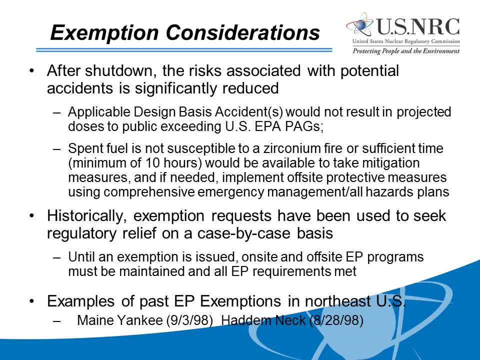 That has a lot to do with part 50. regulations for emergency preparedness do not provide any type of trigger for them to go into a new set of regulations for emergency preparedness. So if they want to get any relief from their emergency preparedness requirements in the 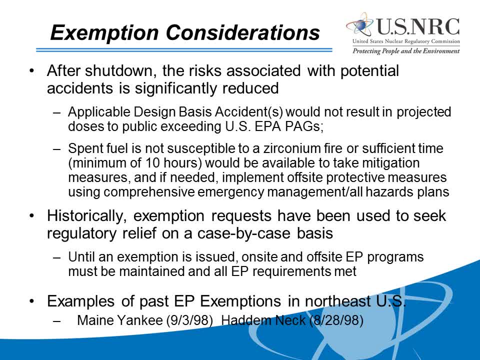 regulations. they have to seek exemptions from us at the NRC. Specifically, they need to seek relief from specific emergency preparedness regulations that would no longer apply to them because of their decommissioning state. The conference has been muted. The conference has been muted. 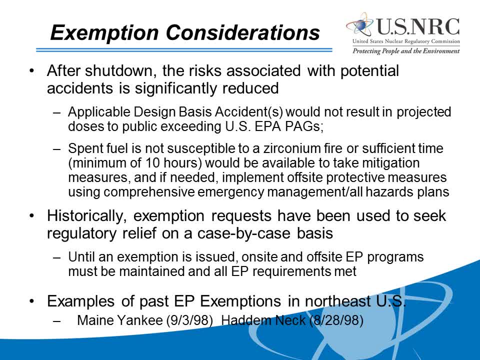 The conference has been unmuted. Okay, Very good, Thank you. I'd just like to remind everybody on the phone that's listening in to please also be on mute. And if your phone doesn't have a mute function, I believe if you press star 69 on your phone. 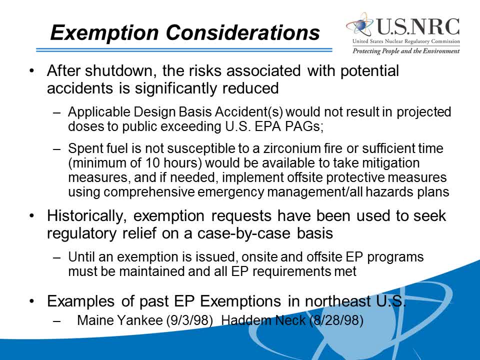 star 6.. Okay, It usually works to mute your phone, even though you may not have a mute button on it. So, at this time, continuing on the considerations for us to give exemptions from the emergency preparedness regulations has to deal with the fact that the risks associated with the 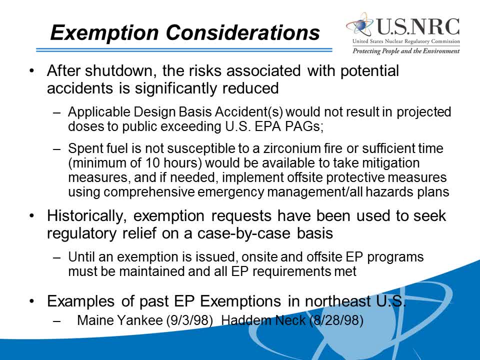 potential accidents that are there for an operating reactor is significantly reduced And that's because the applicable design basis accidents that put in place our plume exposure pathway emergency planning zone, which is normally about 10 miles in radius from the nuclear power plant, those design basis accidents were based on exceeding one REM out to about. 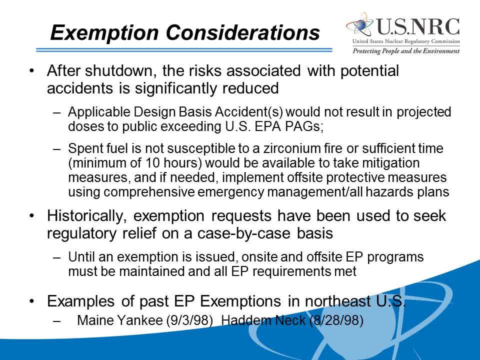 beyond the site boundary throughout that plume exposure pathway exceeding one REM, which would be exceeding the United States Environmental Protection Agency protective action guidelines, the EPA PAAGs. But when you all you have left is a spent fuel pool, with you know, you know, you know. 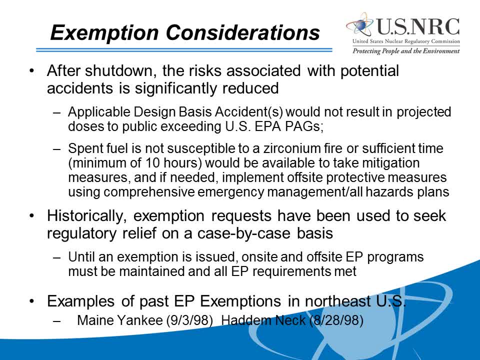 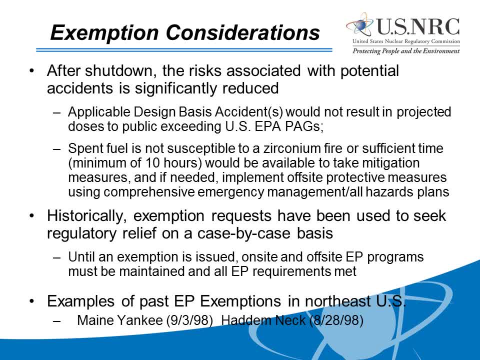 and that's been fuel to provide that. one REM off site to exceed EPA PAG has been significantly reduced And really what is left is the susceptibility of the spent fuel to zirconium fire. And what we do is we ask the licensees: well, we basically say, if you want to get the exemption? 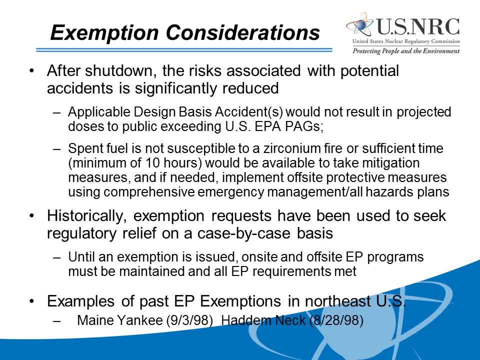 you have to submit to us a spent fuel pool analysis to show to us What the susceptibility is of your spent fuel to that zirconium fire and whether you have sufficient time- a minimum of 10 hours from heat up of the commencement of heat up of the spent fuel- to get to this stage of a zirconium fire. 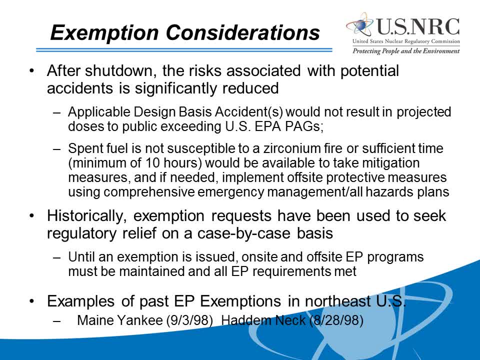 If you have sufficient time to take mitigating actions in order to either do one of two things, and that is to offset the zirconium fire, to mitigate the zirconium fire from occurring, or the ability to implement off-site protective measures, you should have to take action following that event. 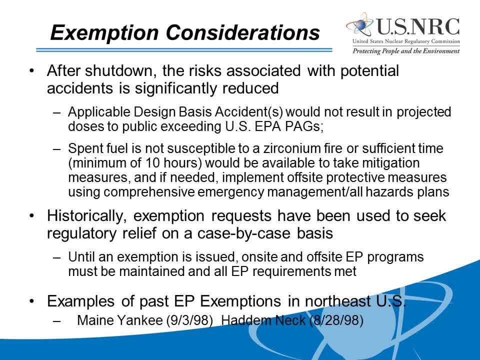 So they send us a spent fuel pool analysis And at that time then we take a look at it And we base our exemption approvals upon that. But until such time they receive that exemption, both on-site and off-site emergency preparedness programs must be met as if they were an operating nuclear power plant with a reactor at 100% power. 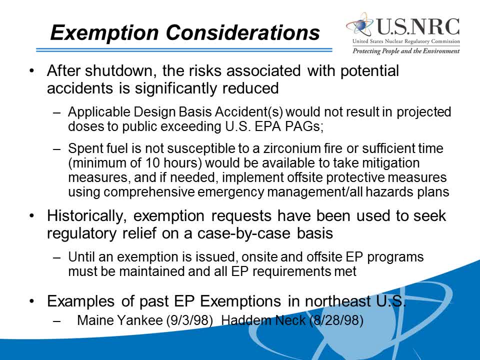 Just to give you some examples, I think Bruce has provided you some past plants. He's talked about those plants that have been decommissioned. The most recent ones are Maine Yankee and Haddam Nest And you can take a look at those to see what type of EP exemptions we provided. 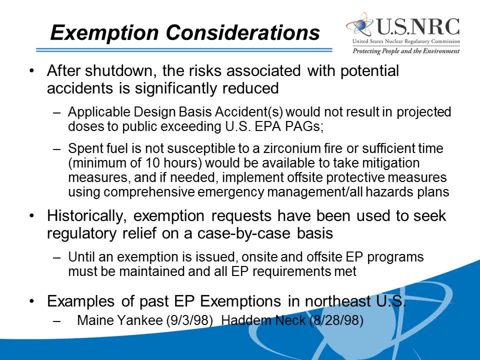 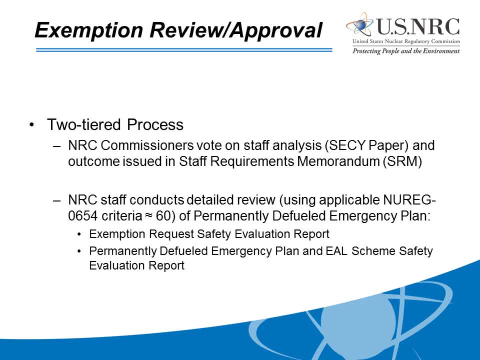 And those are in the northeast United States. But for us to grant that exemption first we have to go through a review and approval process, And it's a two-tiered process. First of all, we put together what we call a safety evaluation report, based upon what they provide to us as far as our spent fuel pool analysis and what they are seeking in exemptions. 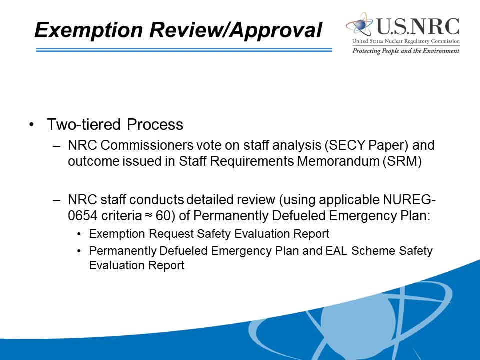 We don't tell them. They put forth to us what they want to seek: exemptions, honor regulations or EP. Once we put together that safety evaluation report, we send a paper- and it's commonly called a SECI paper- S-E-C-Y- up to the commissioners. 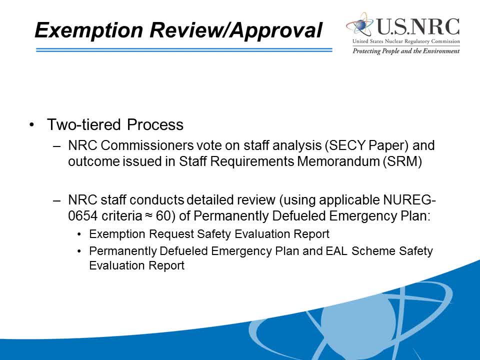 And at the NRC, as you probably know, we have slots for five commissioners, of which four are currently filled, And they vote on our staff analysis in that safety evaluation report And they provide back-up And they provide back-to-us their response as to whether or not they approve or reject our recommendation for the exemption approval. 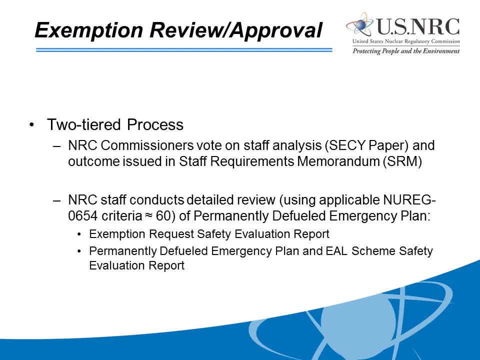 And that's provided back-to-us in a staff requirements memorandum, an SRM. When we do our review and put together that safety evaluation report, we use a guidance document that is commonly referred to as NUREG 0654.. It's actually NUREG 0654-FEMA-REP-1.. 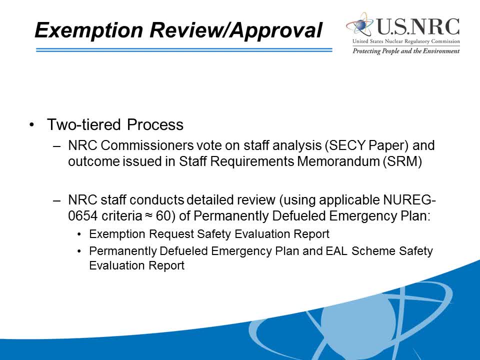 And we take a look at that and we have identified what is it that we would be looking for in a permanently defueled emergency plan, And there's about 60 criteria that are left out of about the approximately 120 criteria- 130 criteria within the document. 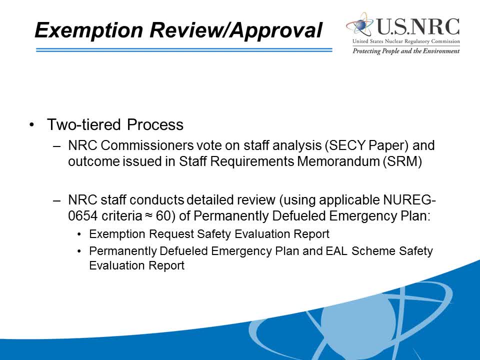 And that's what we take a look at: to see if they have provided us enough justification in their spent fuel pool analysis to warrant their exemptions. At the same time, they provide the At the same time that they have provided us enough justification in their spent fuel pool analysis to warrant their exemptions. 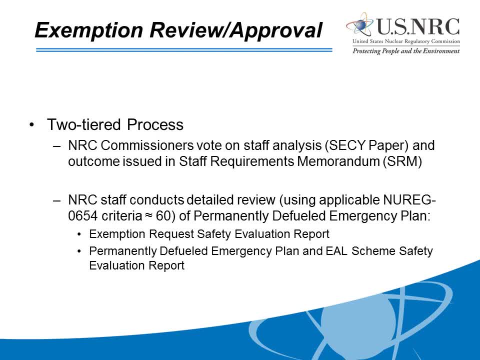 And the adoption of their approx, The Exemption Request to us. We also ask them to provide to us a what what they consider to be a defueled emergency plan. So, once the exemptions are in place, how does their current operating reactor emergency plan morph into a defueled emergency plan? 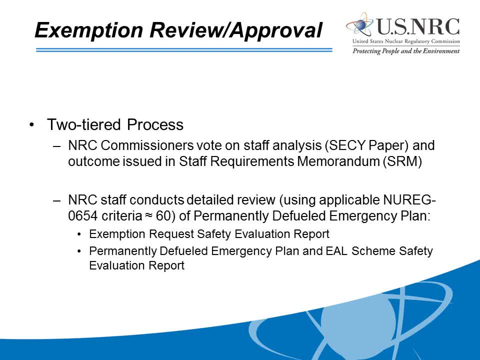 So we have a better understanding about once we grant the exemptions and how they are going to be put into practice within their emergency plan, And also what their emergency action level. That's the EAL Scheme Safety Evaluation Report. We put together a report such that they can change what their classification levels are. 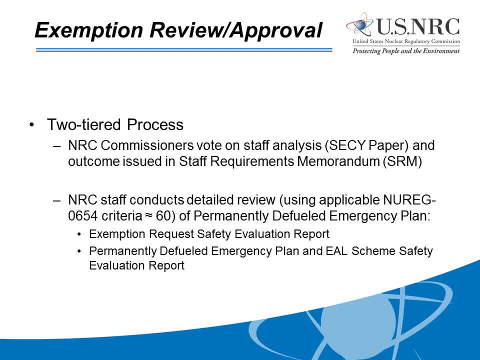 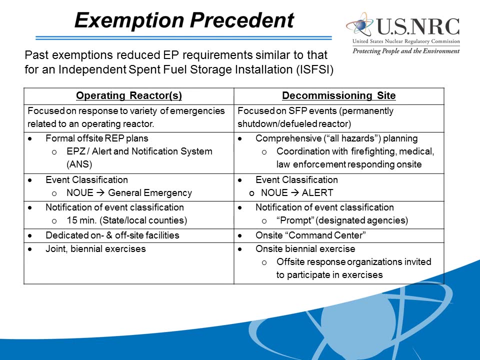 based upon the new suite of accidents, especially the dispensed fuel pool accidents at the site, along with some natural hazards. To give you an idea about what an operating reactor emergency plan, some of the elements and requirements of it, versus a defueled decommissioning site emergency plan is, I provide you this. 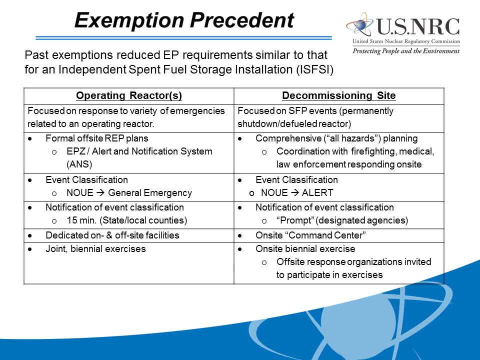 chart and, as you can see on the left side of the chart, in an operating reactor. we are focused mainly on the emergencies related to an operating reactor and then at a decommissioning site. we are mainly focused on the spent fuel pool events such that in an operating reactor. 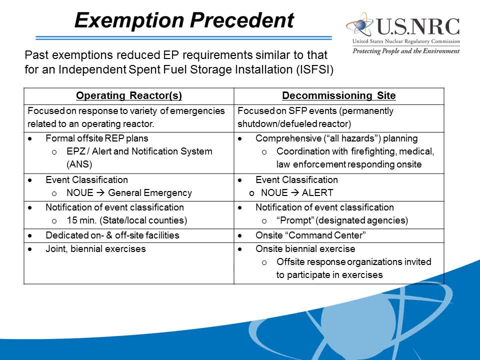 we require that the offsite agencies within the 10-mile emergency planning zone have a formal radiological emergency response plan. FEMA, The offsite agency, evaluates that plan. They are to maintain that emergency preparedness zone with the offsite agencies to ensure that. 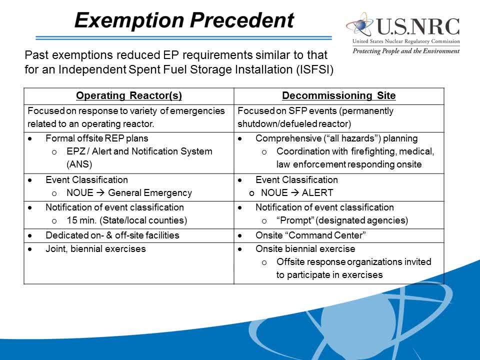 they can take action. They have an alert and notification system. Commonly there are sirens and EAS messages that go over the radio. However, in a decommissioning site, once these exemptions are complete and they go into this defueled emergency plan, there's no longer a need to have formal offsite planning with. 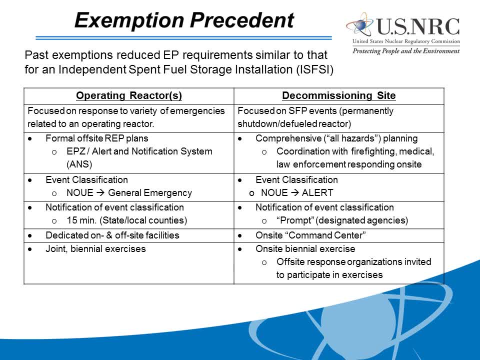 regard to radiological emergency preparedness. This is because, at that point in time, we would have considered that the accident in the spent fuel pool cannot generate a need for offsite response. Essentially, they can no longer exceed one REM at the site boundary and exceed the EPA. 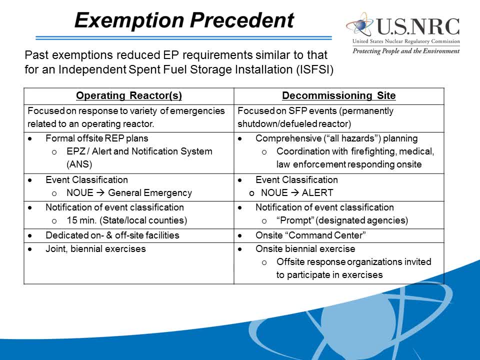 PAGs. So what we are looking for is that the offsite plans need to only be an all-hazards type of plan for response to the power plant, remembering that there is still going to be an offsite response to the power plant. 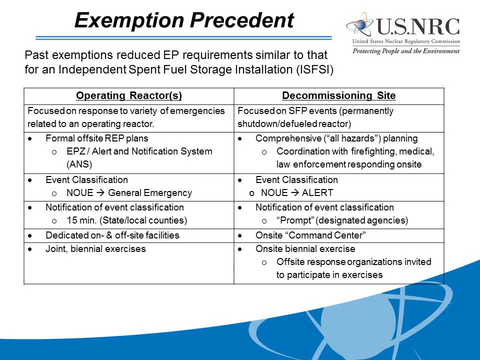 Because it's still an industrial power plant. So it's still going to be an offsite response to the power plant. If it's an industrial facility, it still does have some radiological issues associated with it, but no longer does the offsite need to put into play offsite actions for the public. 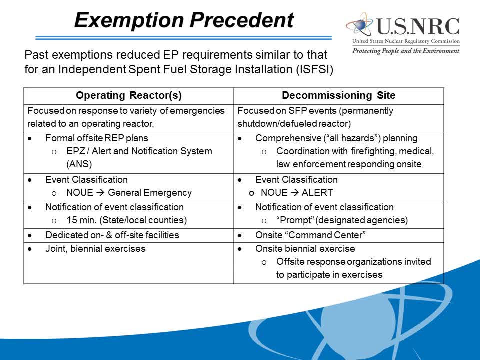 They're looking at how they're going to respond to this industrial facility. Most commonly, we're looking at how they coordinate their firefighting activities, medical activities for personnel at the plant site and, if needed, law enforcement responding if there's a security. 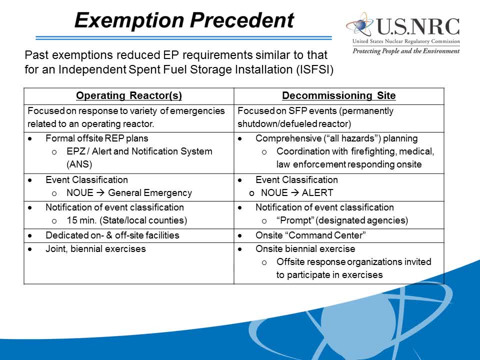 event at the plant site. For event classifications for an operating reactor, there's four levels of events classifications, from the notice of unusual event to an alert to a site area emergency to a general emergency. However, a decommissioning site, you can only get to the alert level and that's due to. 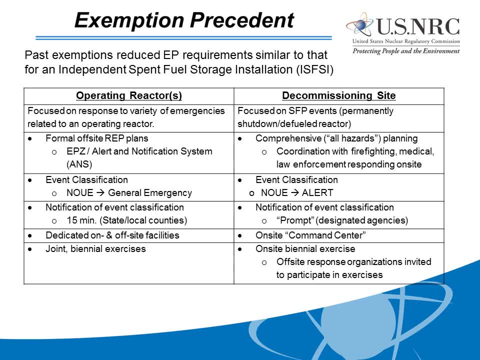 the radioactive releases that can occur. You will not be able to exceed one REM offsite, so the possibility of classifying anything above an alert no longer exists. Notification of events for an operating reactor: 15 minutes to the responsible state and local. 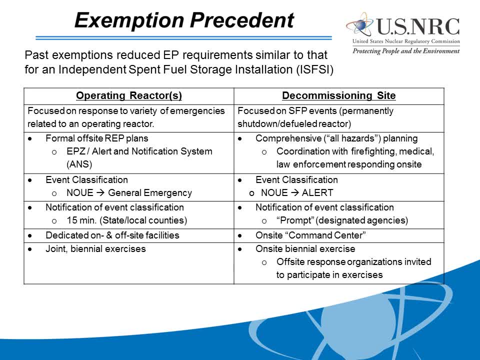 county response organizations, but for a decommissioning site we only require them to have a prompt notification. What we have been seeing actually for all exemption requests we've had for all of the decommissioning sites, is they prefer to go from a 15-minute to a one-hour notification. 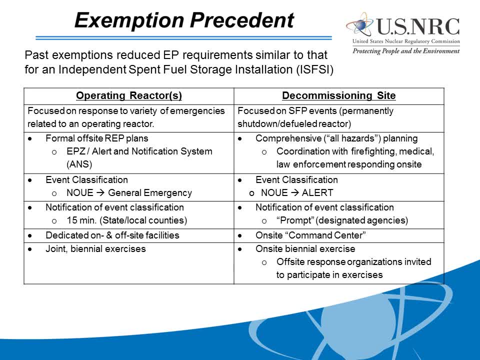 And that is because really there's no need for an offsite response. It kind of puts the offsites into a monitoring mode in case they would need to respond offsite for any type of events and mostly for public relations and such. 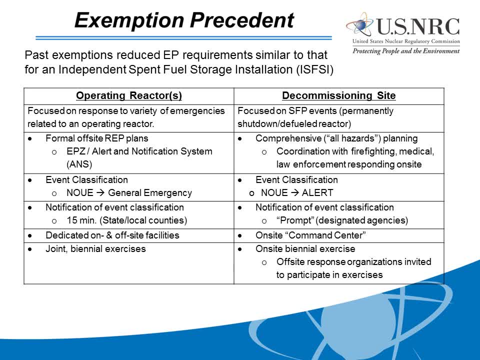 For operating reactors you need a dedicated on and offsite facilities for emergency response. Most commonly on site you see a technical support center and an emergency operating facility And for the offsite agencies they'll have an emergency management agency. Emergency agencies will stand up their emergency response facilities. 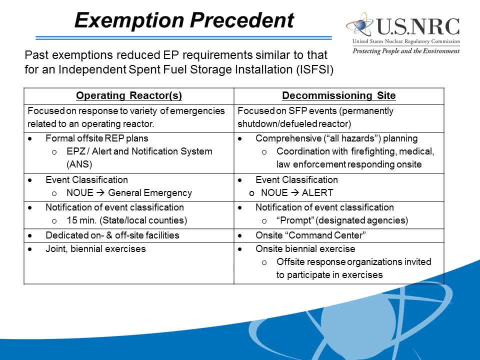 But for a decommissioning site you won't have any of the offsite facilities being required any longer. But traditionally what has happened is they transition from these formal type of emergency response facilities to essentially a command center where they can group people in in. 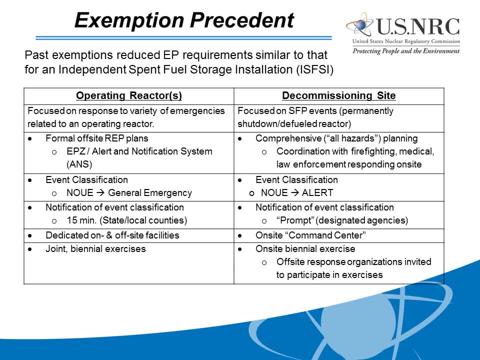 order to respond to an emergency And for an operating reactor, you have a bind, your exercise requirement, where they must hold an exercise once every two years with offsite agencies and it is an exercise where they jointly conduct a radiological emergency response, which would include the need to provide 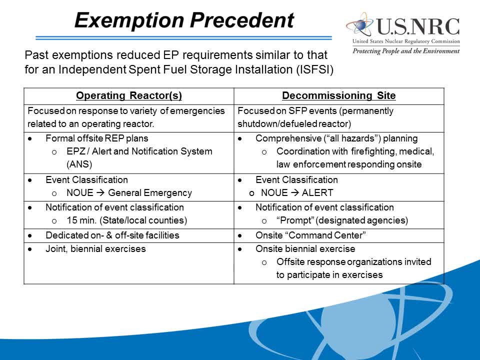 protective actions for public. But for a decommissioning site the removal of the requirement for offsite participation occurs And at that point they still have to do an offsite. We have an on-site portion for responding to an event on site, but the offsite response 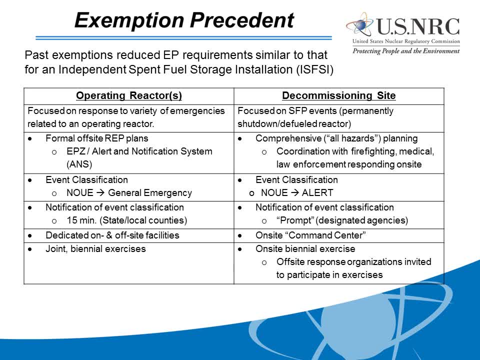 organizations are only invited to participate in the exercises and a lot of our decommissioned sites still do that because they still want to know how they can coordinate with a fire response ambulances coming on site or the need for law enforcement. 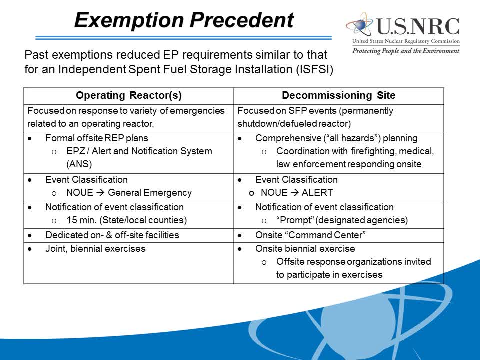 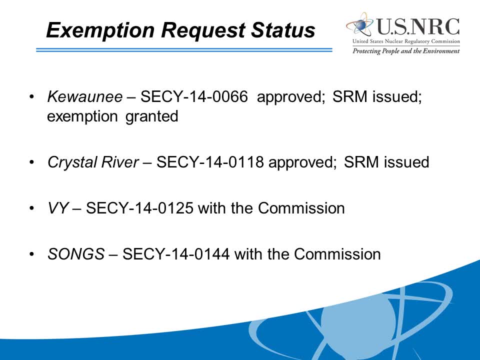 So exemption request status and this is for the most recent Power plants that have gone into decommissioning status since January of 2013,. Kewaunee, and this is the SECI paper, as I said, a paper sent up to the Commission. 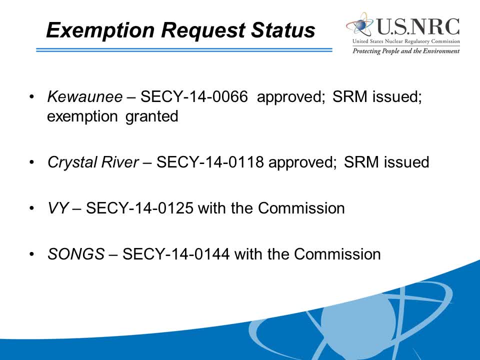 You can see what exemptions were recommended by the NRC for the Commission to approve. That was in SECI 14-0066, and that SRM was issued and the exemption was granted. Crystal River- That SECI paper. The SECI paper went up earlier in 2014, and the Commission came back with their staff. 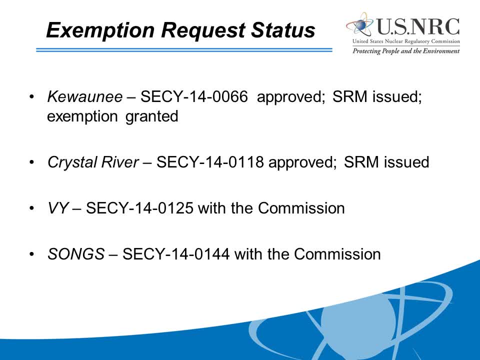 requirements memorandum granting those exemptions And also for Vermont Yankee and Song's. this slide was provided for this presentation early last week and in the meantime those two plant sites, Vermont Yankee and San Onofre Nuclear Generating Station, the Commission has provided us. 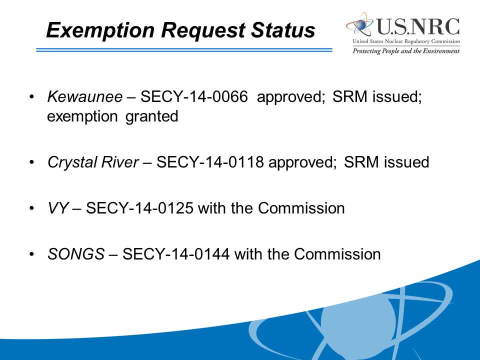 A staff requirements memorandum, and both of those sites have also gotten their exemptions approved. So all four sites now have exemptions approved in the area of emergency preparedness. We're just waiting now to send out the letters to tell them they can start to implement their 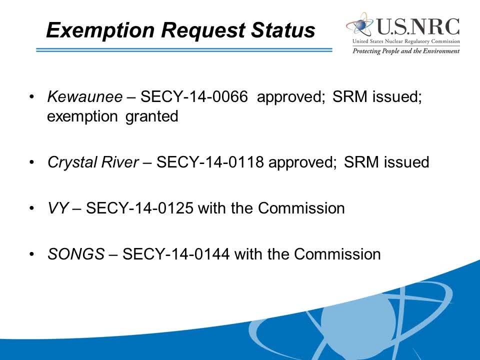 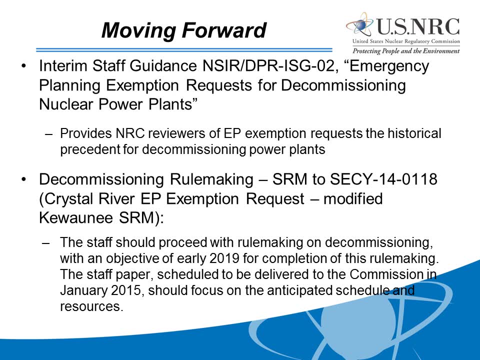 permanently defueled emergency plan. Moving forward, we have put together what we call an interim staff guidance document, the emergency planning exemption request for decommissioning nuclear power plants. We're going to talk about that later, Thank you. Thank you, Chris. 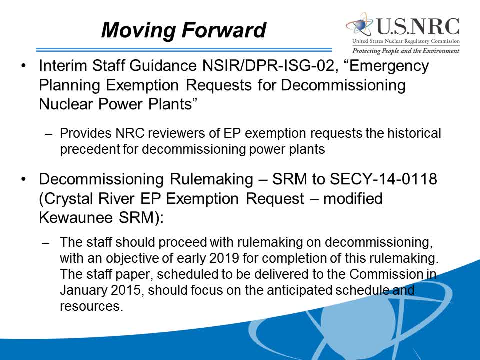 Thank you Jim, Thank you Crystal, Thank you all, And we're going to move on to the next slide and we're going to talk about the emergency preparedness. So we've got a little bit of a preview here. 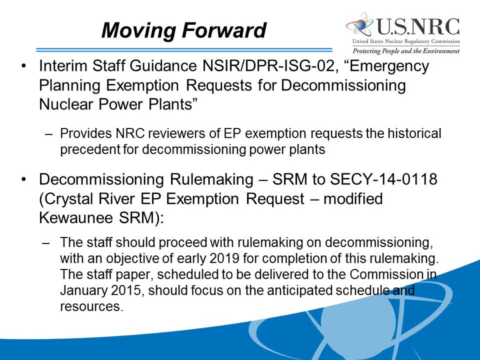 There's a little bit of a preview here. We've got some of the things that we talked about in the previous slides. The first thing I'll say is that we're going to be not only doing some of the review and then the review, but also the review of our emergency preparedness, and we're going to 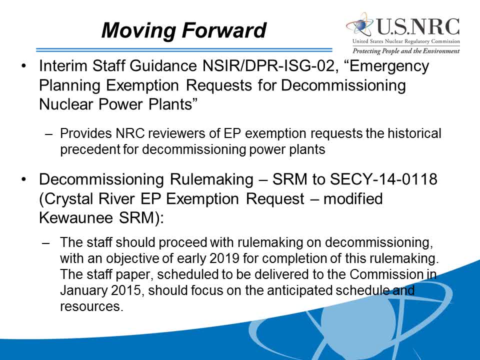 take a look at what we can pull out of it. We'll take a look at what we can pull out of it. We're going to take a look at what we can pull out of it. Well, instead, what we've decided to do was to provide guidance document out to the licensees. 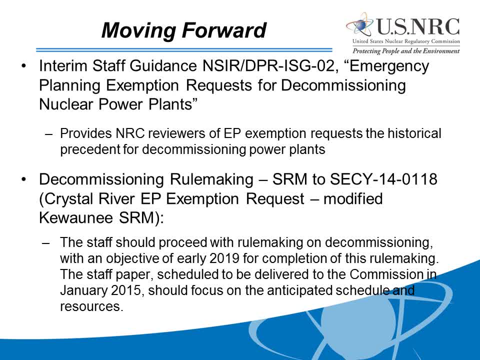 also for own internal use, on how we are going to handle exemption requests with regard to emergency preparedness, and it was based a lot upon the historical precedent for the for the decommissioned power plants that were done prior to 2013 and that this interim staff guidance document is planned to be. 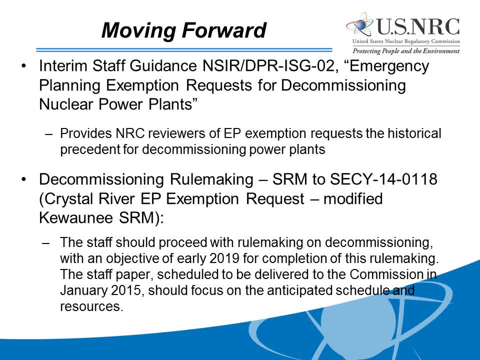 issued. you know you may not see it, but keep my fingers crossed, hopefully by the end of this month, that it's not the end of this month of mid-april, so it will be coming out and all nuclear power plants in the future will at least have some. 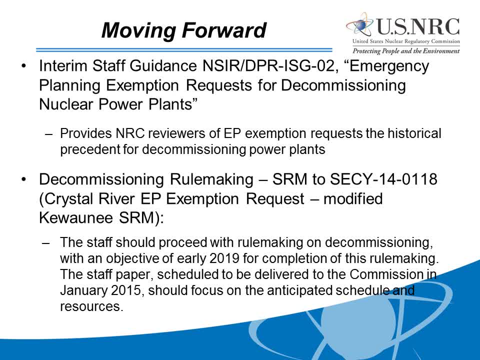 sort of guidance on and how to put together their exemptions and what would seem to be acceptable to us, as long as they provide adequate justification. in the meantime, when the Kewaunee staff requirements memorandum came down granting approval of their exemptions, that was in August of 2014- the 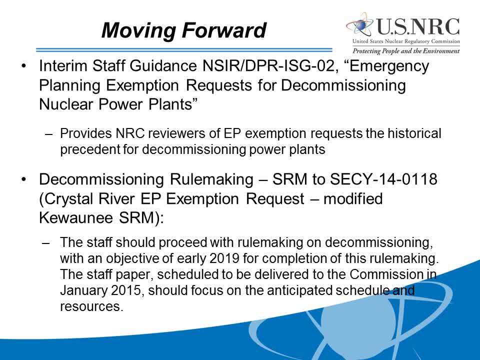 Commission had directed the staff to to consider doing rulemaking in the area of decommissioning and in one of the specific topics was an emergency preparedness. there are some other areas but emergency preparedness is definitely one of those to be considered and we are to respond back to Commission in January. however, when the Crystal River emergency 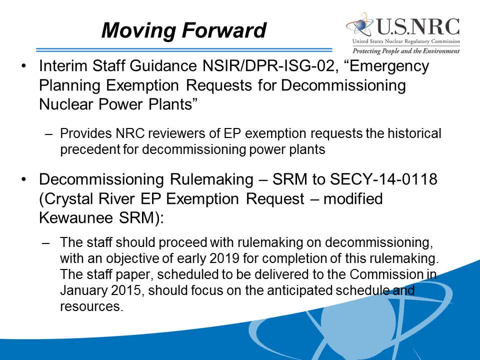 preparedness exemption staff requirements memorandum came back late December of 2014. it modified the previous staff requirements memorandum to say- not to tell us- whether we would consider it. the Commission then directed us to initiate the commissioning rulemaking with an objective of having it completed by early 2019, and we are now in the throes. 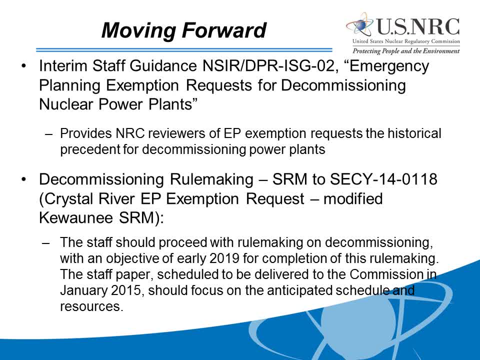 of beginning the process of determining how we're going to proceed with that rulemaking and putting together a schedule and resources and provide that back to the Commission in the next few months. so by early 2013, 2019- excuse me- there will be decommissioning rulemaking hopefully in place for emergency. 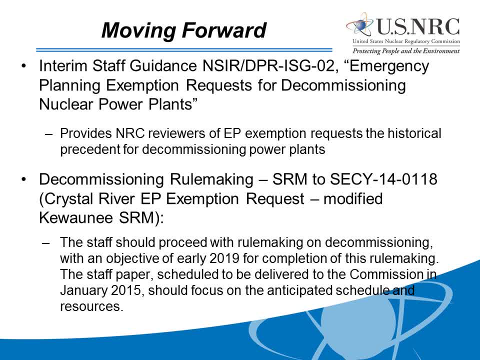 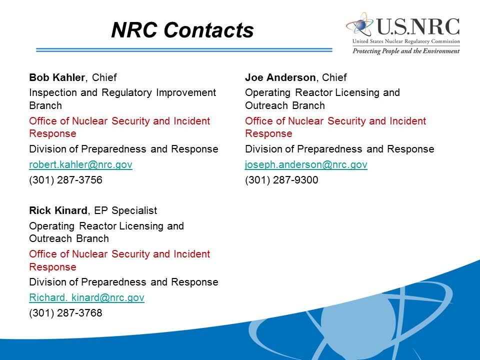 preparedness, security and some other areas for for sites that will be commissioned following that time. with that, I'd like to give you a few contacts within answer: our office nuclear security incident response, and these are strictly contacts for emergency preparedness. my own contact: there, Joanne, I'm the guy that's going to be doing the leading the. 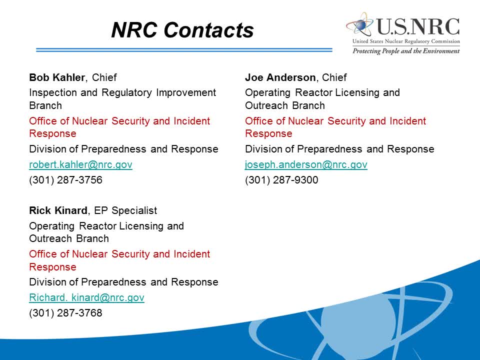 charge on the decommissioning rulemaking. with regard to emergency preparedness, Joey Anderson is the individual who is in charge of reviewing and approving the exemptions that are provided by nuclear power plants, and Rick Kennard of our group, is the individual who is working closely with FEMA to make sure that, as 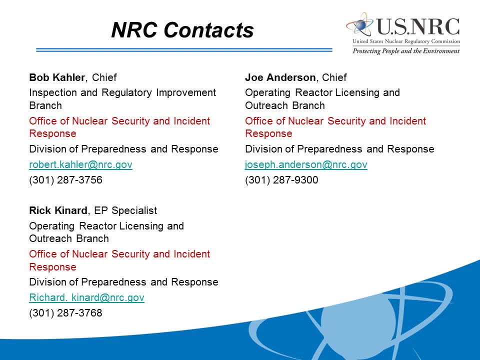 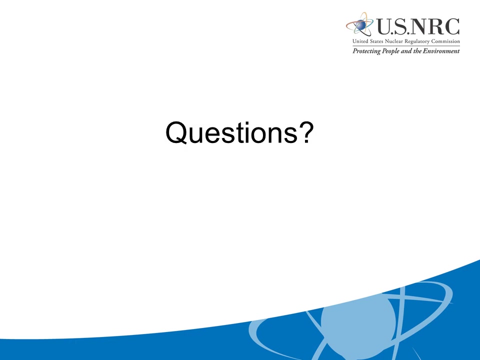 we, as we grant our exemptions to nuclear power plants and removal of off-site responsibilities, that FEMA is an alignment and can take action off-site and aid them in making the transition. so at this time I think Bruce and I are both done with our presentations and we can open up to questions. great, this is, Meredith. thank. 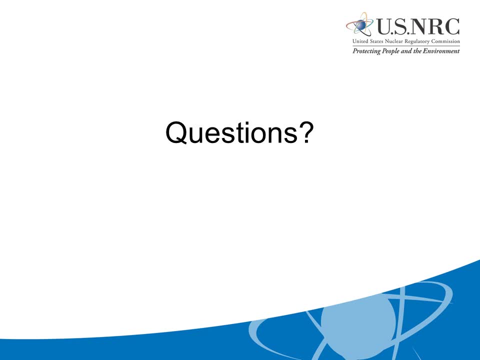 you so much for those presentations. they were great, very informative. if you have a question, please feel free to ask. if you'd also like to ask over the chat feature online, I will read your question out loud. so do we have any questions for the presenters? you 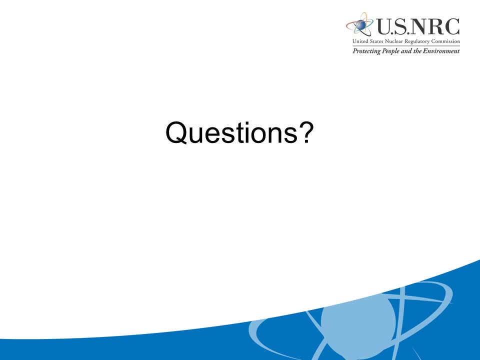 great well hearing done. I'd like to thank you all so much for presenting today and I also like to thank you all for joining our webinar. it will be archived online and if you have any other questions, please feel free to contact the presenters or myself or the NAR and a. 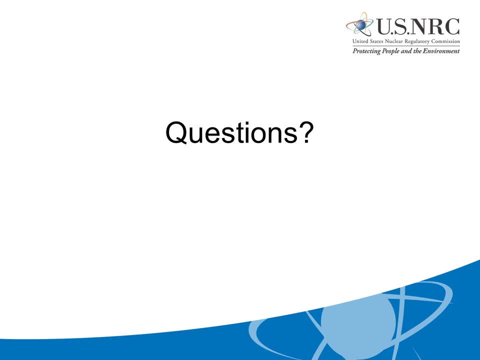 copy of the slides, would hope. if you are able to log on to the NAR website in the next few weeks, we'll have the entire webinar archived, so you'll have the slides as well as the audio. thank you again, and I appreciate your time this afternoon. Meredith, I just saw a question pop up in the chat. ah, okay, great, we have. 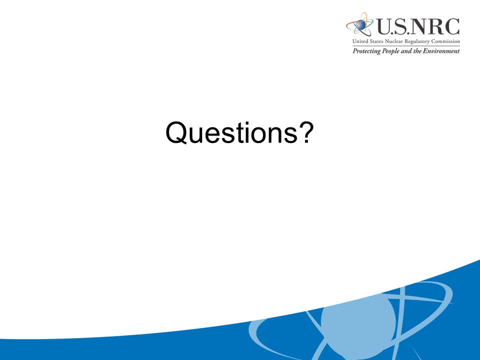 one from Stephen Helmer and the answer is say that 25 miller per year decommissioning criteria doesn't include all pathways and the answer is yes, 25 miller per year plus Alara includes all pathways. so that would include the groundwater soil resuspension, the amount in the soil, amount on building surfaces. 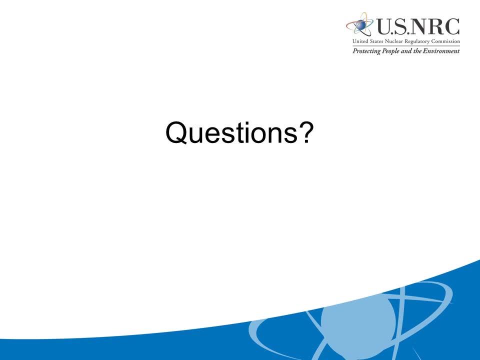 if they're still building surfaces, their ingestion of the water, ingestion of any plant materials grown, they're going into the food supply, etc. etc. so, along with the common ingestion and inhalation. so the answer is yes, great, thank you. any other questions before we adjourn? all right, well, thanks very much and I hope to see all of you sometime soon in. a upcoming meeting.